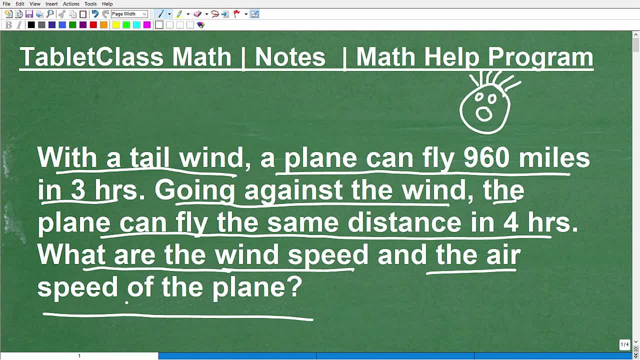 Sometimes the wind's going with us and sometimes the wind's going against us, So that's going to obviously influence the amount of time it takes us to get to a particular location. So I'm going to break all of this down in just one second, But first let me quickly introduce myself. My name is 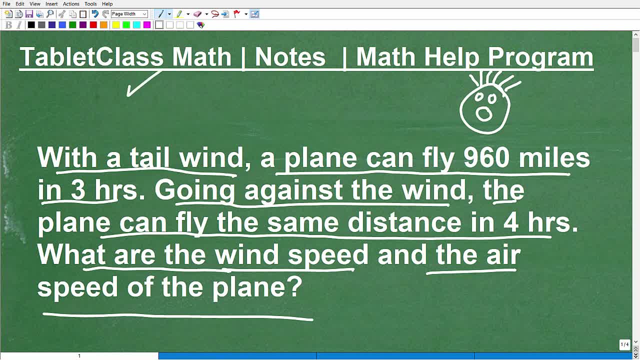 John, I'm the founder of Tablet Class Math. I'm also a middle and high school math teacher And over several years I've constructed what I like to believe is one of the best online math help programs there is. Of course, I'll let you be the judge of that. If you're interested, you can check. 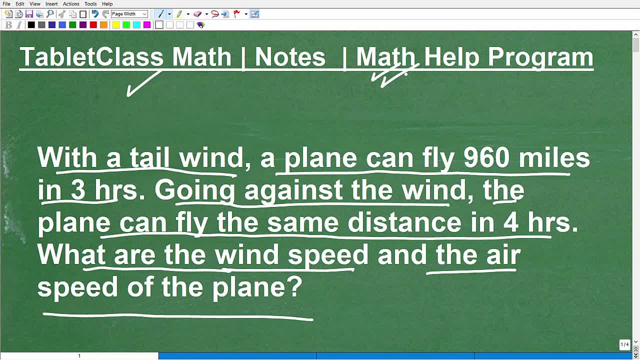 out my math help program by following the link in the description of this video. But basically I have 100 plus different math courses. I have all the main courses, like pre-algebra, algebra 1, geometry, algebra 2.. I'm going to be launching pre-calculus here. 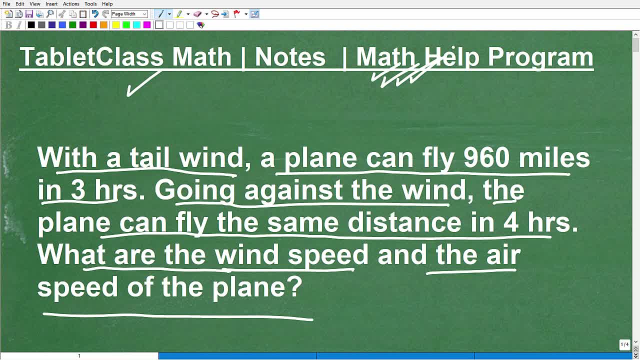 shortly, But I do a lot in the area of test preparation as well. So if you're preparing for the GED, HiSET, maybe the GRE, GMAT, ASVAB, CLEP exam, ACCUPLACER, ALEKS, SAT, ACT, Let's see here. 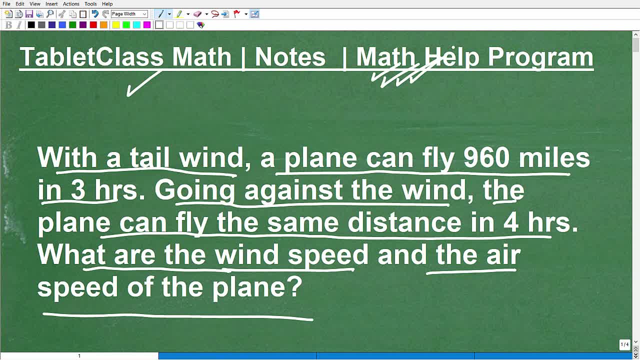 Maybe a teacher certification exam, maybe a nursing entrance exam, maybe a teacher certification exam, maybe a nursing entrance exam, maybe a nursing exam. All those exams I've mentioned have significant math on them, As a matter of fact, more than just basic math. some of those exams have pretty advanced math, And if you don't get 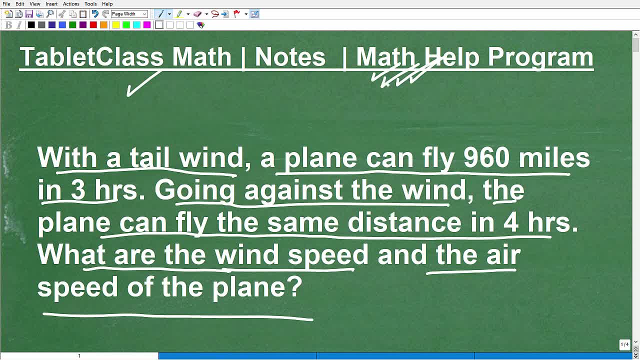 to the math section on these exams. you don't pass those exams which have negative consequences for your goals. So I can definitely help you out. Just go to my site, check out my full course catalog And if I don't have the exam you're preparing for, drop me a line and I'll help you out the best. I. 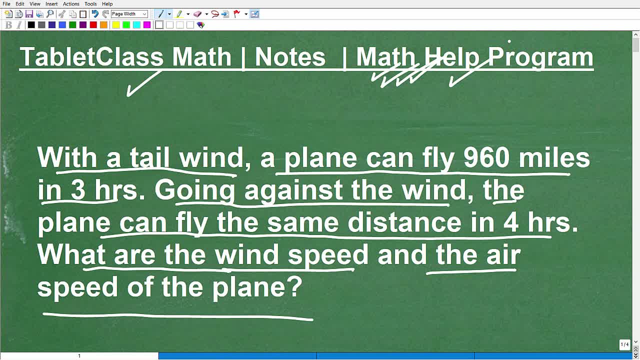 can. I also do a lot with independent learners, like homeschoolers. So if you homeschool, I got a great homeschool program. And then, lastly, help those of you that are just struggling in your math class. Okay, so it could definitely help you out. But one thing I can't do for you that you must. 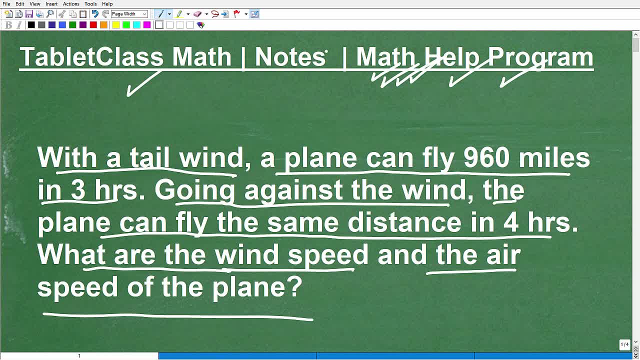 do for yourself if you're serious about improving in mathematics, and I assume that you are. if you're watching this video, that is the following: Okay, you have to take great math notes Over decades of teaching mathematics. it just appeared to me. 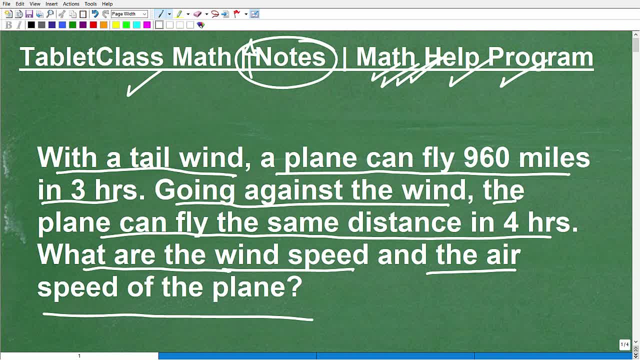 those students really take the time and effort to take great math notes, almost always do well Okay. and the reverse is true. Those students are just too busy looking at their cell phone, talking to their friends and doing homework for other classes while you're in math class. well, don't be surprised that you know you're struggling. 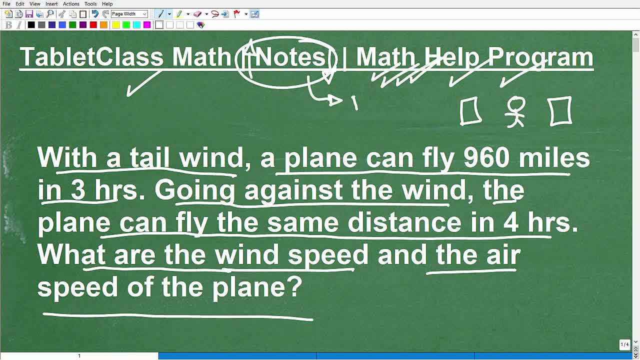 Okay. so you got to focus to learn math. there's no other way, There's no shortcuts and it is work. But if you put in the work and you're focused and engaged, guess what, For the most part, all of you out there are going to do very, very well, okay. But 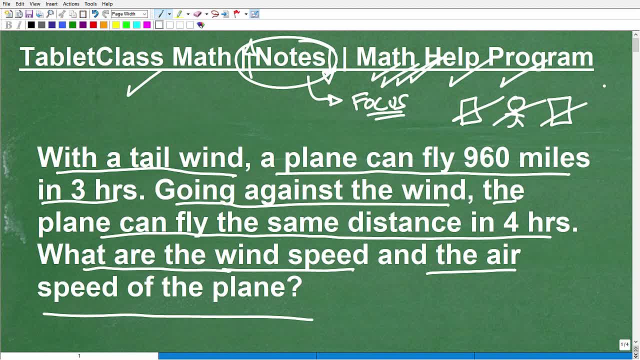 if you do any of these things, I'm not trying to make you feel bad, because I was definitely distracted way back in the good old days of the 1980s in class. Of course I didn't have a cell phone, and I'm glad I didn't, because if I had a cell phone I don't even know if I would have. 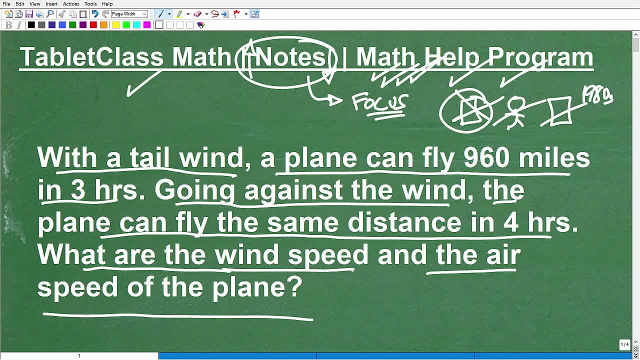 graduated because I would have been completely distracted. So it's a lot of work to stay focused, but it's up to you, It's your own responsibility to do so, So no other activity is better than note-taking to force you to stay focused. okay, So definitely work on your notes, but as you're 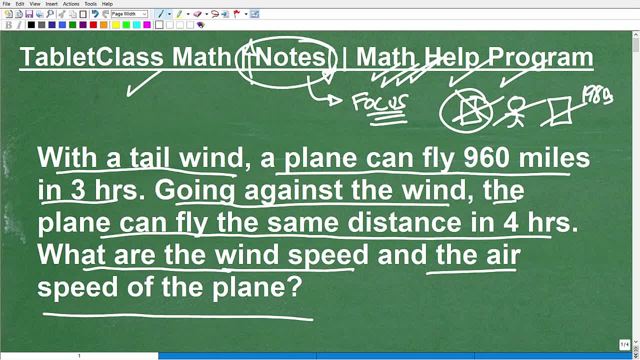 doing that, you still need something to study from, So I offer detailed, comprehensive math notes to include pre-algebra, algebra 1,, geometry and algebra 2, and trigonometry. You can find links to those notes in the description of this video. Okay, so here's our problem. Obviously, if you 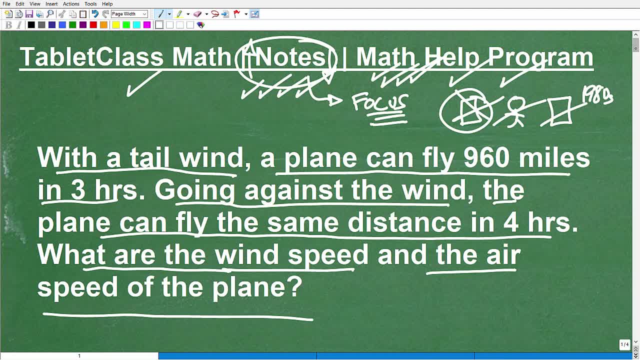 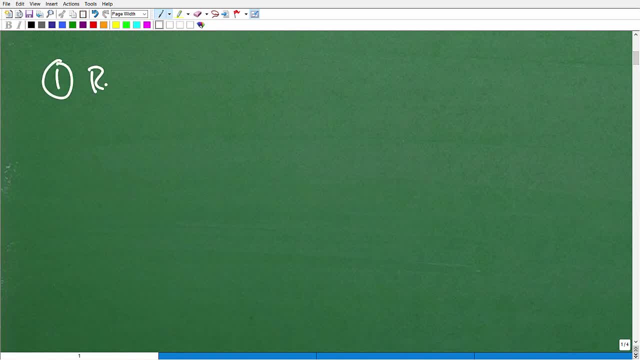 want to try it. Go ahead and pause the video and give it a whirl, but let's just quickly talk about the main steps to solve an algebra word problem. So the first thing is you want to read the problem. Now some of you are out there like saying, okay, that's kind of obvious. Well, no, that's not what. 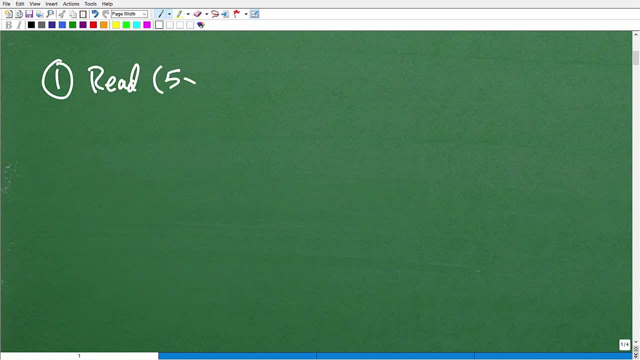 I mean okay. I mean you need to read the problem, like at least five times. So don't just read the problem and then start doing math. You shouldn't go into a word problem like that. You want to read it, get a feel for what's going on. and then you're going to get a feel for what's going on. 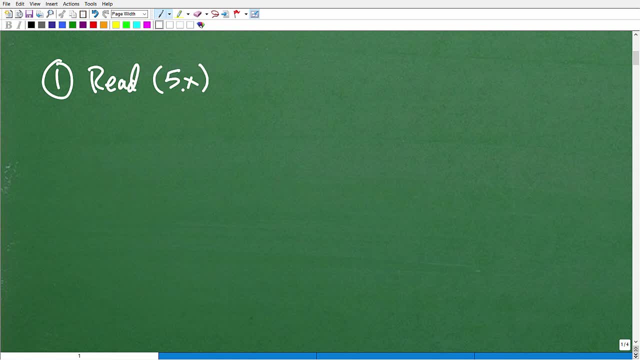 And then you're going to have to reread it and read it again, read it again to continue to pull information out of the problem. So don't ever just read the problem once and then go Okay, so you're going to have to read, read and read and read. Okay. so that's the first thing. Now the second: 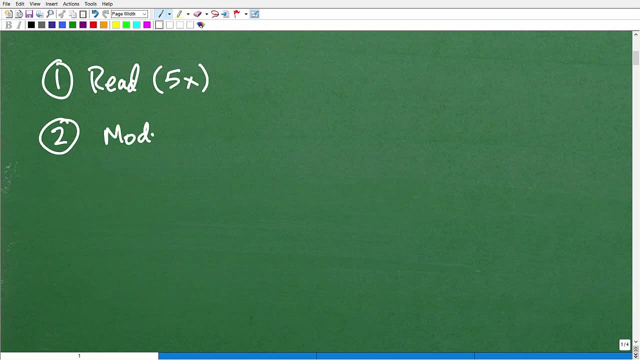 thing is, you want to create some sort of model. all right, Some sort of. it could be some sort of sketch, It could be some sort of table, It could be something, but try to model the information. that's in the problem. 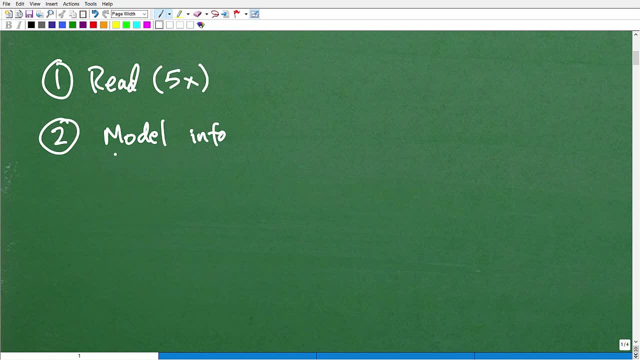 Okay, so this is really, really important. all right, So it could be. stylistically, it could be different for different students, but you just don't want to go from you know the actual words and the prompt to like an equation, right? You try to construct some sort of model. It's going to be. 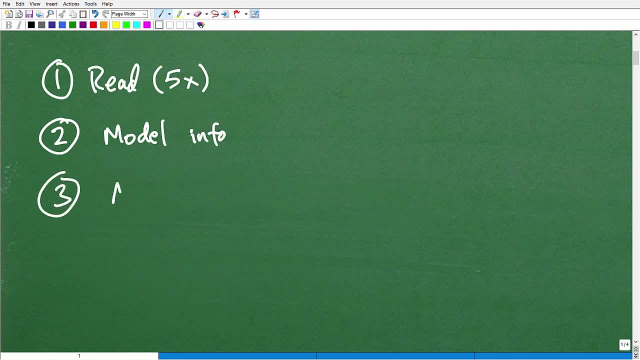 very, very helpful. Now, the third thing is you need to assign, okay, some variables- variable or variables, It all depends on what the situation applies. but you need to say, okay, we're going to let x equal to this, all right, or let y equal to that. So you know, we are doing algebra here. so 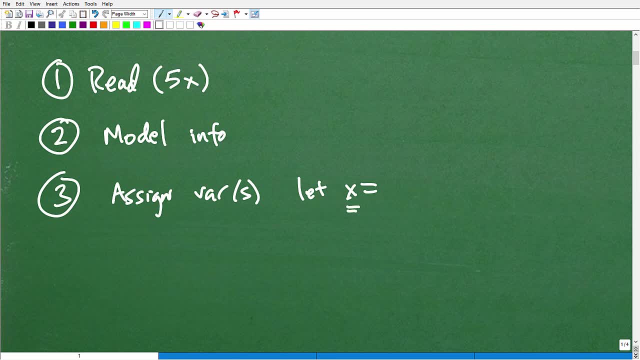 if you're going to, you know, assign a variable, you got to be clear on what that variable represents. Oftentimes it's going to represent the unknown value that you're trying to solve for in the problem. Now, the fourth thing is you want to, once you've assigned variables and you kind of modeled, 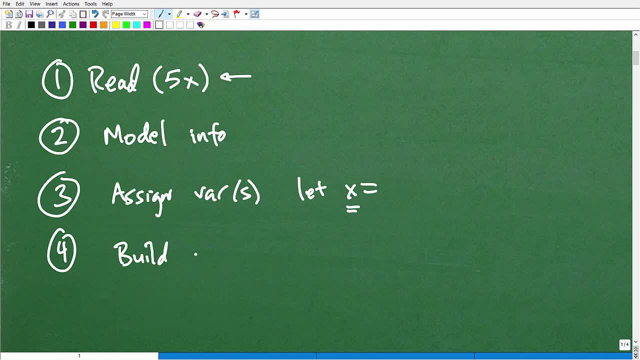 information. you want to try to build some sort of model, So you're going to want to assign a variable to some sort of equation. okay, some sort of equation or equations, all depending on the type of problem that you're dealing with, and it's going to involve, obviously, the variable that you have assigned. okay. 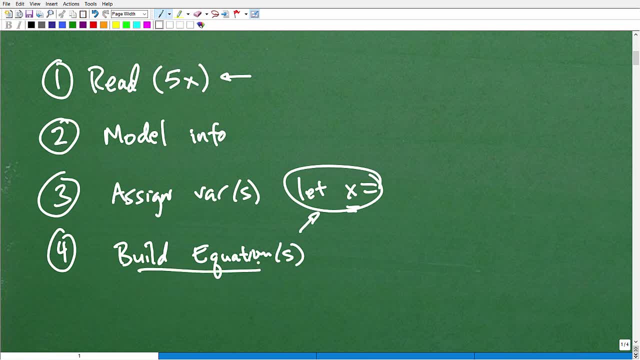 because you can't solve for a variable unless you build some equations. Now, when you're building equations, you need to look for relationships, and this is where knowing basic formulas- okay- come into play, and the formula that we're going to be using in this particular example is going to be: 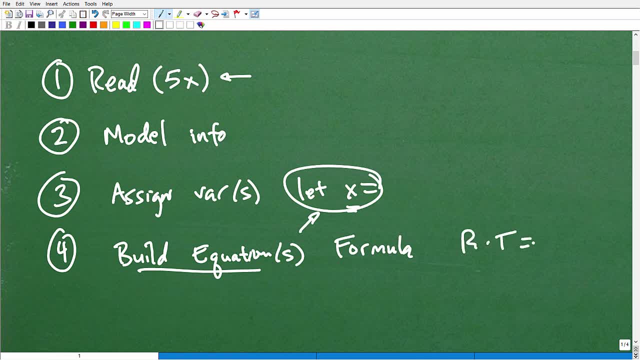 is rate times time is equal to distance. This, right here, you should know. okay, it's a basic in basic algebra or math students. so rate times time, speed times time, is equal to distance. You should be familiar with this formula. If you're not there it is, We're going to use it here in. 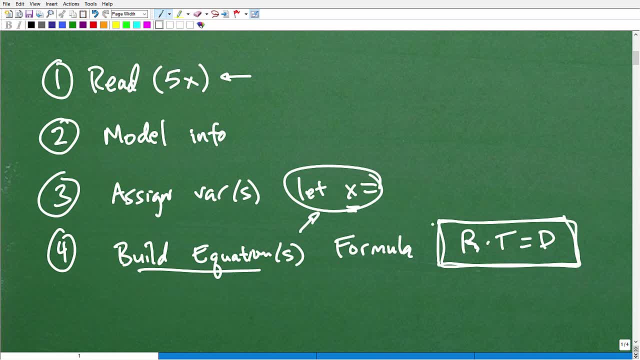 a second, but this is a big one and there's other basic kind of formulas here. So again, this is just a general overview of the steps you want to take in an algebra word prompt. So you're going to build equations Again when you're. 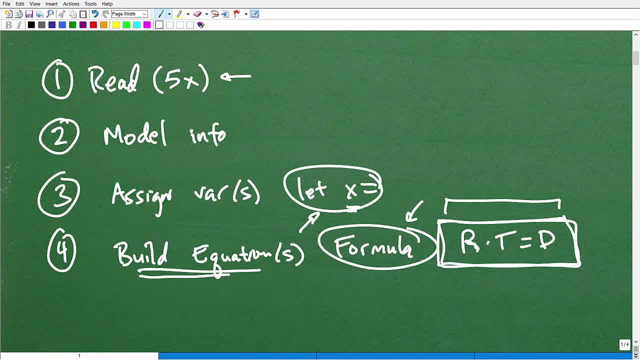 doing that, you might be using a formula, because a formula has some sort of relationship between variables. right, All right. so the next thing you're going to do is you're going to solve your equation, or equations. okay, Now, at this point a lot of students think they're done. Oh, 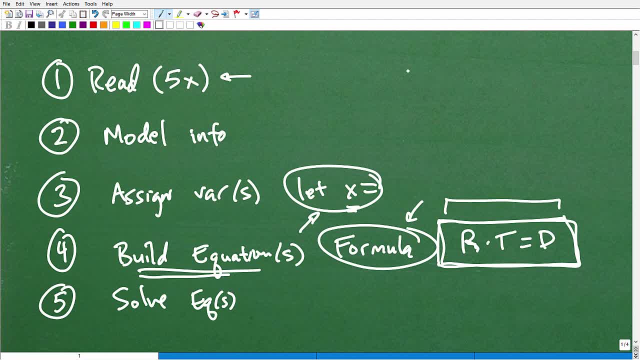 I solved the equation. I'm done with the problem? Nope, not exactly. The sixth step is you need to solve the question, okay, So oftentimes when you solve these equations, you may have to do one or two additional steps to actually solve or answer the question asked in the original prompt. So 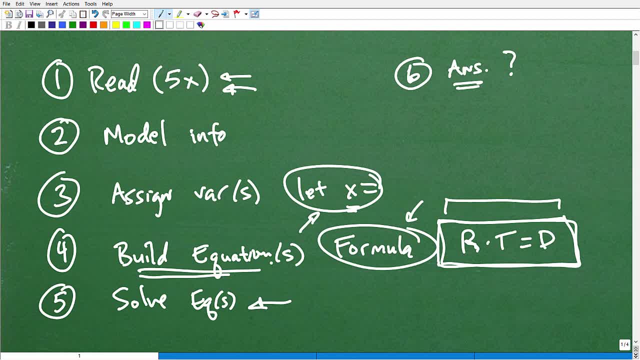 you're not done until you say: okay, what did I just solve for? Let me reread the prompt again, make sure that I have the correct answer and then answer the question right. So this is a basic model for word prompts. Now let me just say right now that I have other videos. 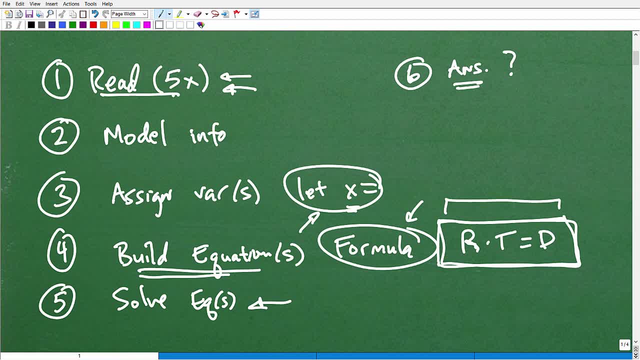 in my YouTube channel, in my pre-algebra and algebra playlist, I think even my algebra 2 playlist on word prompts. So you could practice more word prompt problems by going to those particular videos, if you like the way I'm breaking things down so far, Okay. so now I'm going to go. 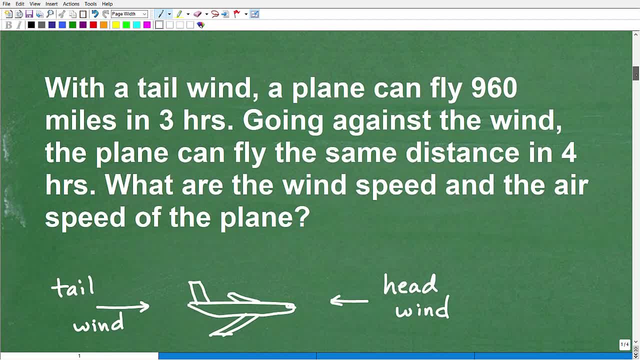 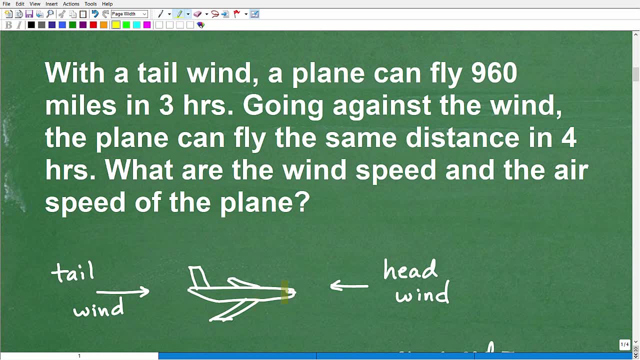 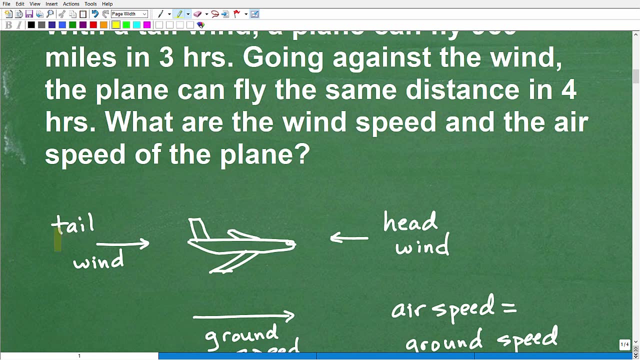 ahead and get into this problem, All right, so let's read it again. So with a tailwind. now let's just make sure we understand conceptually what a tailwind is. So here's our airplane, It's in the sky, So we're talking about a tailwind and a headwind here. So a tailwind is, if you're. 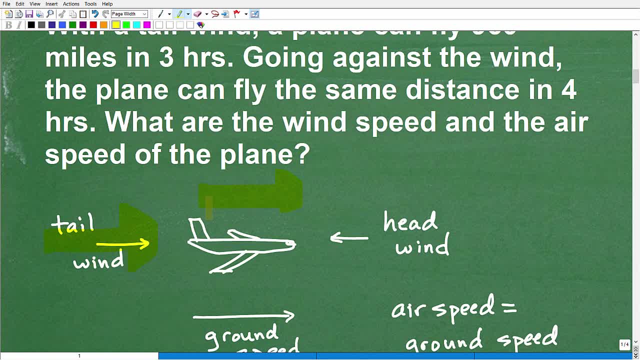 going this way, it's wind that's behind us, So is it going to make the airplane go faster or slower? Well, obviously it's wind to our back, So this is going to make the speed of the plane faster. Likewise, if here's my airplane and I got wind blowing, you know, into the airplane. 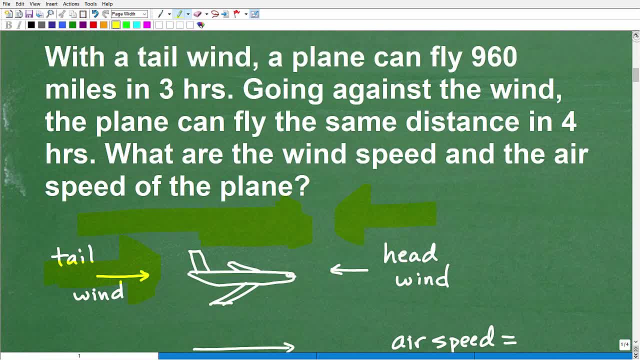 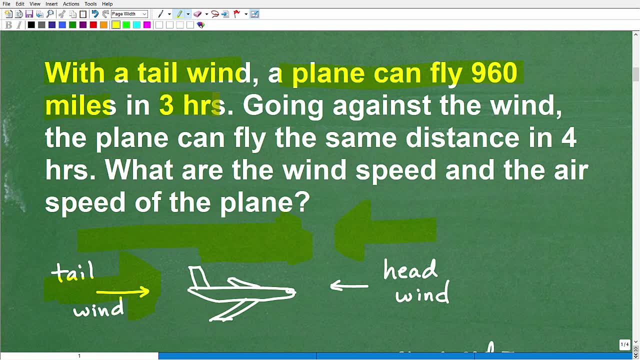 it's going to slow it down, So we just need to have some basic idea here. So with the tailwind, a plane can fly 960 miles in three hours. Okay, Now, going against the wind, that would be called a headwind- The plane can fly the same distance in four hours. So 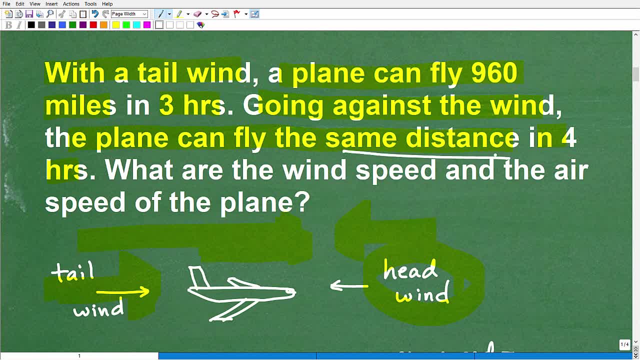 we're talking about the same distance here. Okay, So that's interesting. And what is that distance? It's 960 miles. Okay, All right, So with the tailwind, okay, obviously the airplane goes faster. It takes three hours, Okay, To do this. 960 miles, And with the headwind it takes. 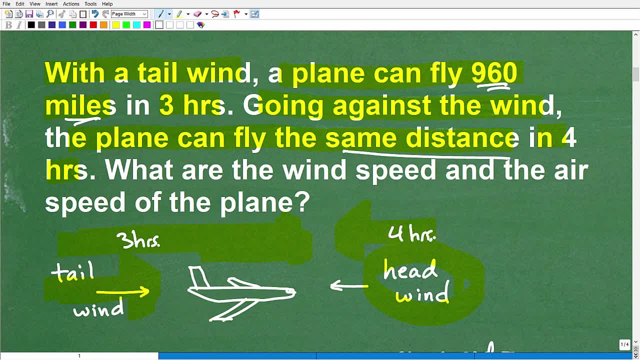 four hours. So here's kind of like a basic model, some sort of sketch, And then we want to answer what? What are the wind speed? Okay, So here it's the speed of the wind, And then what is the? 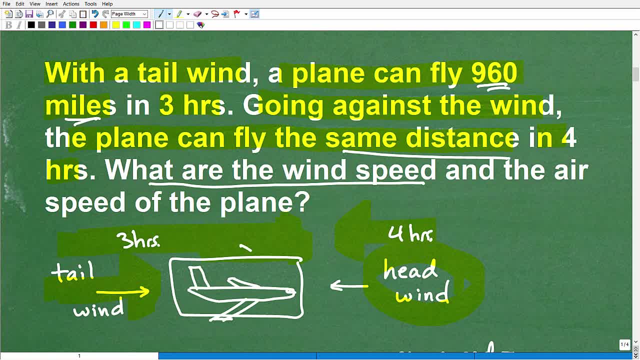 airspeed of the aircraft, Because the aircraft is going at a particular speed, Okay, And then we have this wind speed that's either slowing us or making us go faster or slowing us down. Okay, All right, So that is the problem. 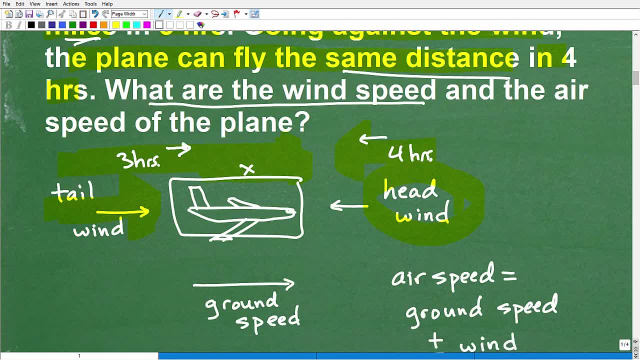 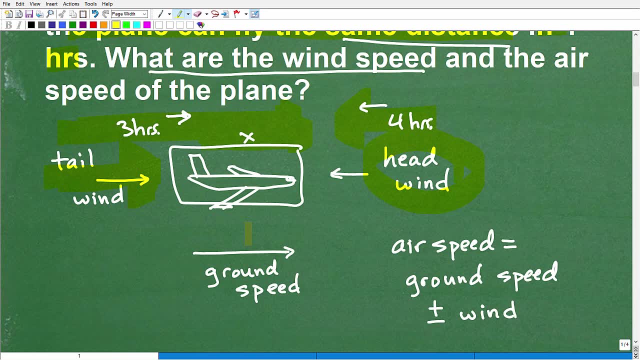 Now, of course I'm going to refer back to the problem as I build out my equations here, But this is my. you know, this is what I'm talking about: building a model or sketch, something like this. So you kind of see what's going on Now in algebra, once you learn how to do one style. 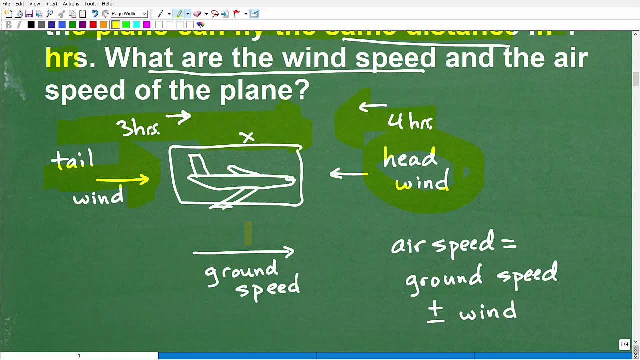 or problems. this is, these are what we call motion problems, So you can kind of see what's going on. Okay, So once you get this problem down, you'll see other similar problems like it. So in that, especially in basic algebra, algebra one, there's kind of a variety of problems. 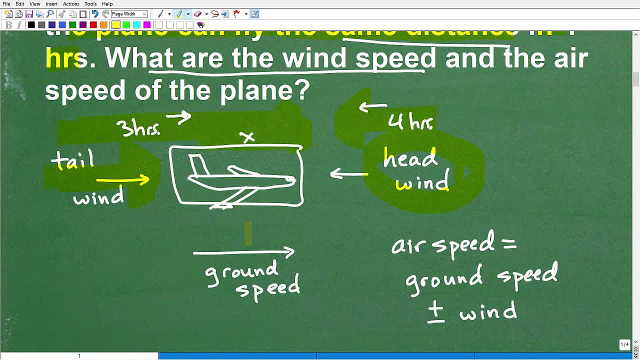 common type of word problems that if you understand how to solve one, you'll be able to solve others. Okay, So, again. so the airspeed, all right, is going to be the ground speed of the airplane, plus or minus the wind speed, depending on how you build the model. So 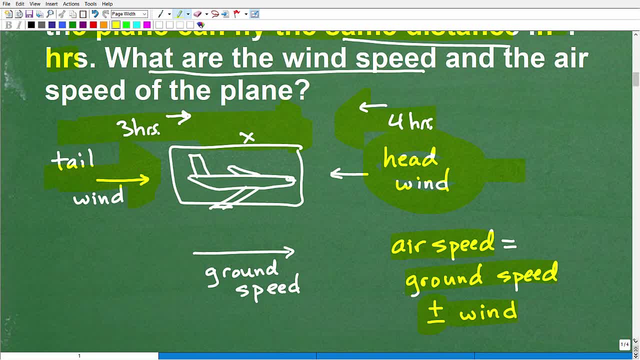 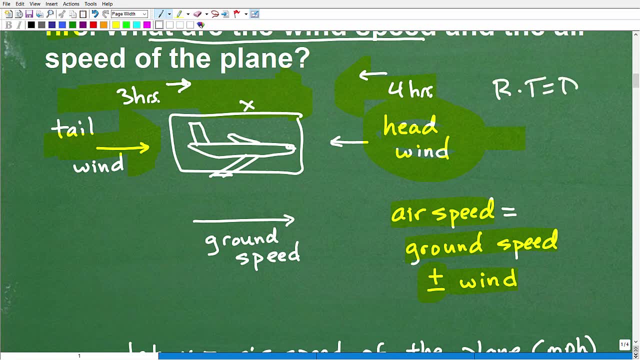 whether it's a headwind or tailwind. okay, now remember that other formula that I said that we're going to be using. so rate times. time is equal to distance. rate is what rate is speed? if you didn't know what that is time? okay, it's. 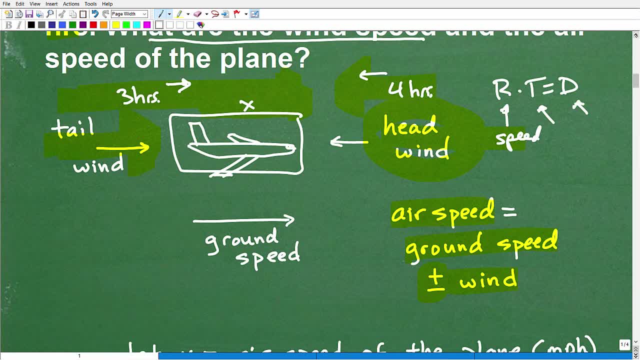 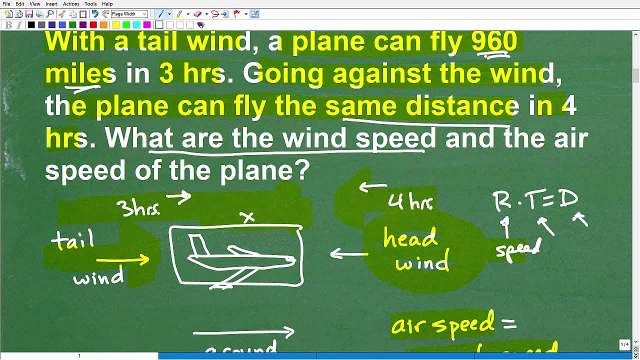 obviously, time and distance is things like what we have right here, like miles, right. so one thing we want to be careful about is: okay, we're talking about rate times. time is equal to distance. our distance is measured in miles, okay, so this is important. our time has been given to us in hours, okay, so our speed? 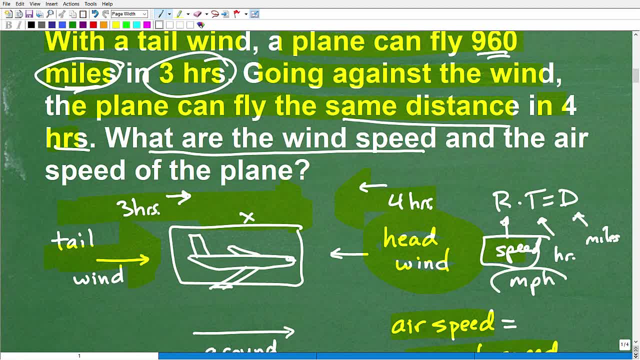 is going to be miles per hour. okay, miles per hour because I'm dealing with miles and hours. so you got to be careful with the units of measure. again, in this particular problem we don't have to do any convert conversion, but you may have to do converting units of measure in other problems. okay, again, I. 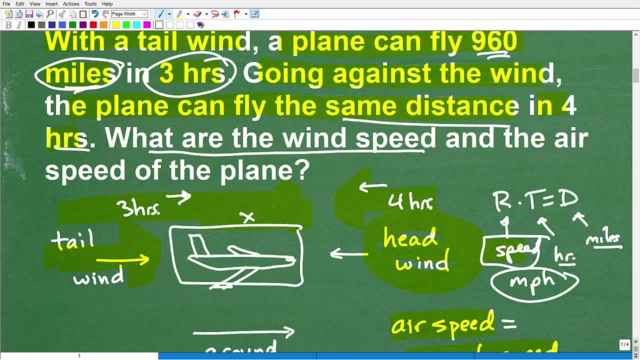 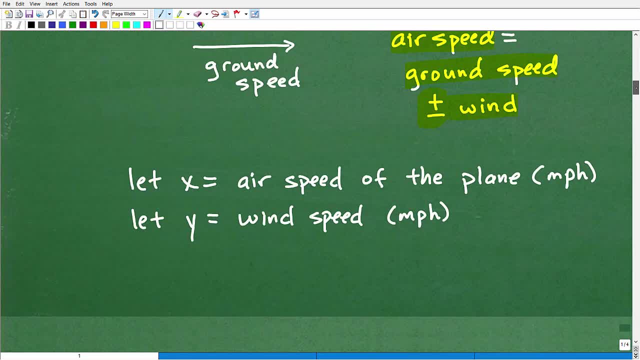 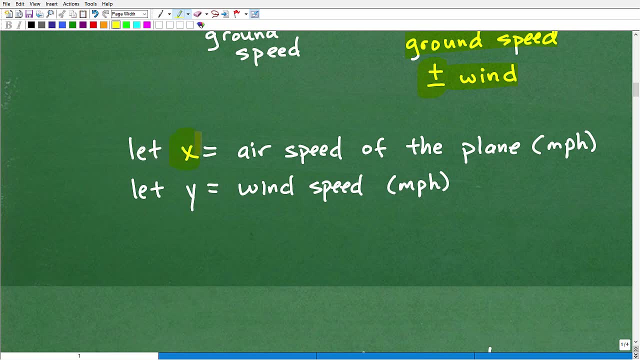 have other videos, other word problems. you can check those out in my playlist. but let's get to this problem here. all right, let's keep going now. the next thing is let's go ahead and assign some variables. so I said: let's let X- we'll choose this variable X. let's let X equal the airspeed of the plane in miles per. 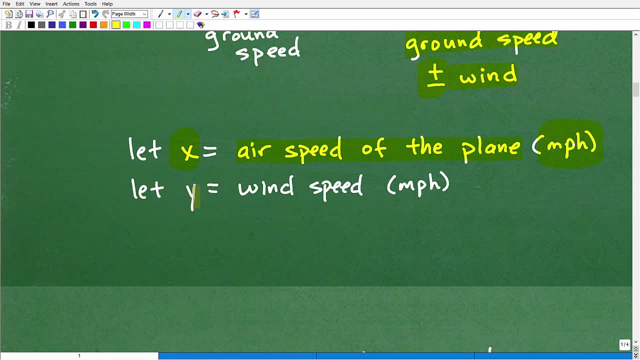 hour. again the speed, we're dealing with miles per hour, and then we'll let Y okay be the wind speed, okay, so the wind. so let's just kind of like be a little bit more precise with what's going on. so the airplane is going from here to here, okay. so here's the plane. it's going like so. 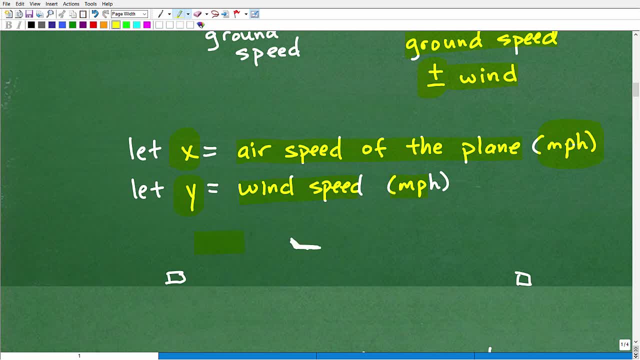 all right, now the wind could be like this. all right, it's gonna be going at some mile an hour. so, as the plane is going from here to here, it's in, the wind is in this direction. it is what it's. this is the tailwind. this is when it does it in three hours. right, because it's faster. 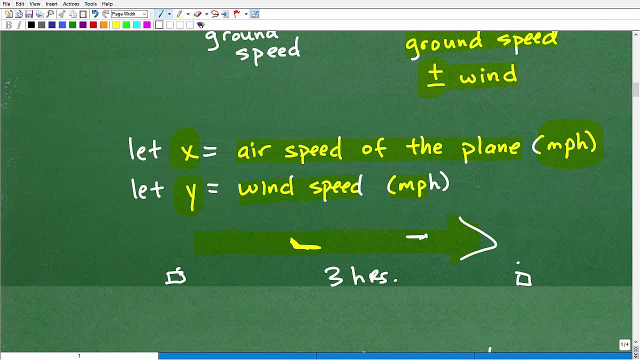 but the wind is still in this direction. so when the airplane returns, it's doing it in four hours. okay so, but the wind speed is so constant and it's in one particular direction. so here's our plane on its return trip, and now it's going against the wind, but the wind, again, is going to be at one speed, so we could. 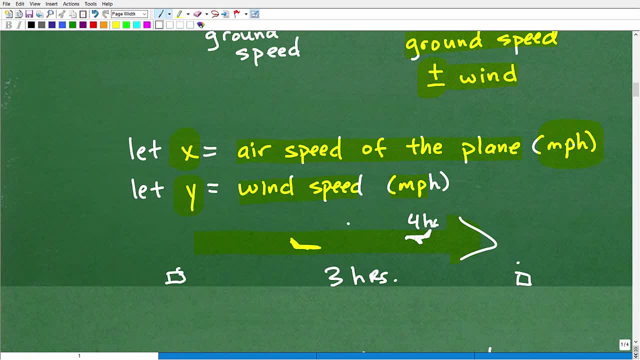 just say: okay, let's let Y equal the airspeed of the plane in miles per hour, Y be equal to the speed of the the wind, and then we'll let X be equal to the airspeed. okay, all right. so that's basically the two variables that I have. 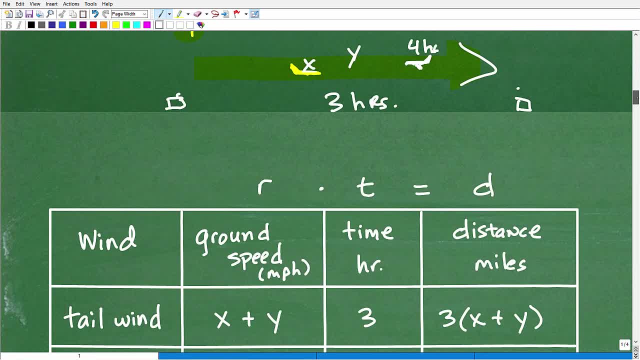 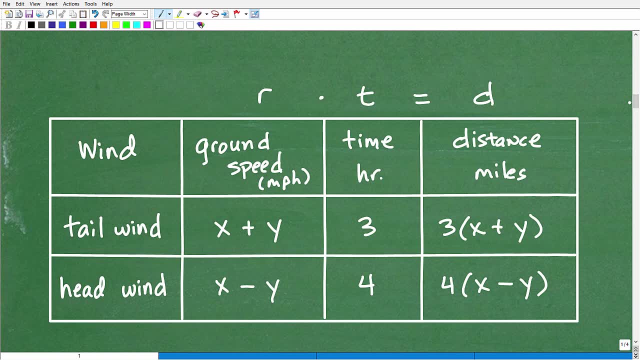 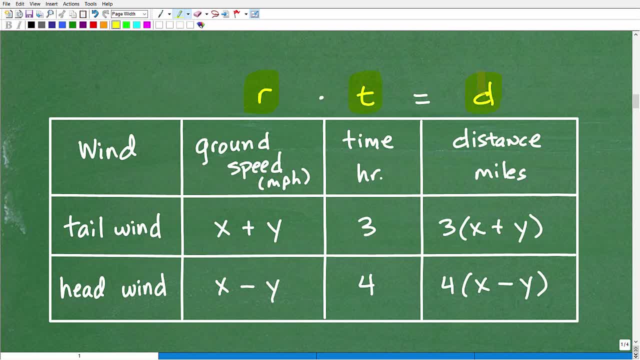 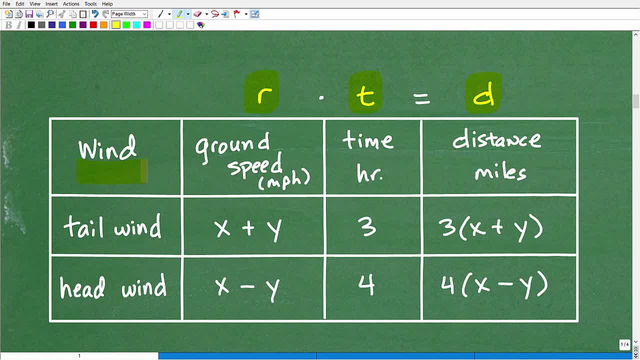 times, time is equal to distance, but let me show you how I broke this up. so what do we got going on here? well, we have. do we got going on here? well, we have. do we got going on here? well, we have wind we have to have, we have to consider. 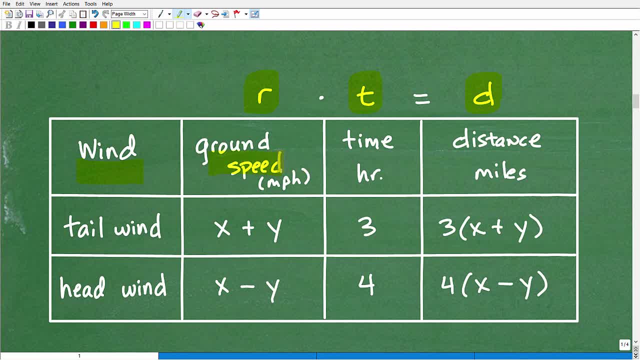 wind we have to have, we have to consider wind we have to have, we have to consider the wind, and then we have the ground, the wind, and then we have the ground, the wind, and then we have the ground speed of the aircraft. okay, now the speed of the aircraft. okay, now the. 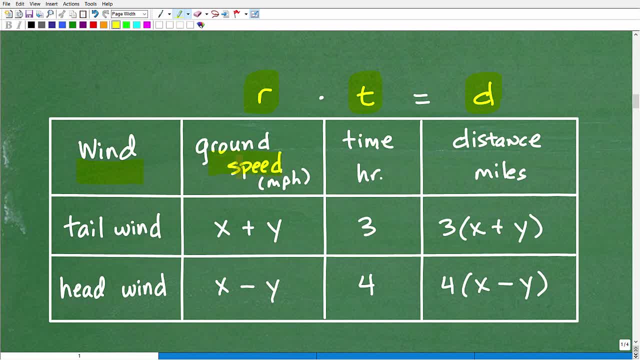 speed of the aircraft. okay, now the ground speed would be like the actual ground speed, would be like the actual ground speed would be like the actual speed. it's flying okay, like how fast it's speed it's flying okay, like how fast it's speed. it's flying okay, like how fast it's flying okay, like how fast it's going to get the flight. and then we have 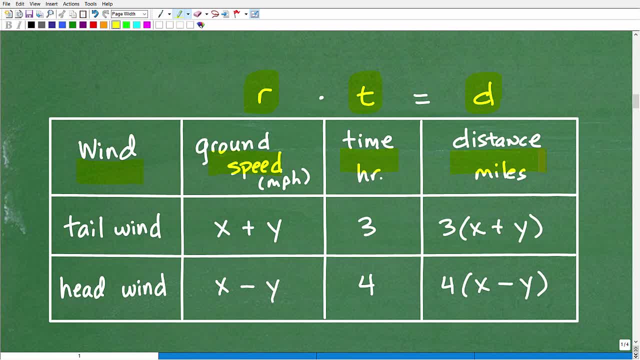 flying okay, like how fast it's going to get the flight, and then we have flying okay, like how fast it's going to get the flight, and then we have the distance the airplane traveled all going to get the flight, and then we have the distance the airplane traveled all. 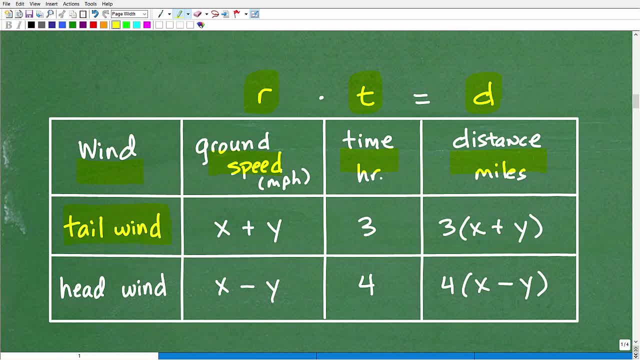 going to get the flight. and then we have the distance the airplane traveled- all right. so let's take a look at this one: the distance the airplane traveled- all right. so let's take a look at this one: the distance the airplane traveled- all right. so let's take a look at this one situation. we have a tailwind, so the tail. 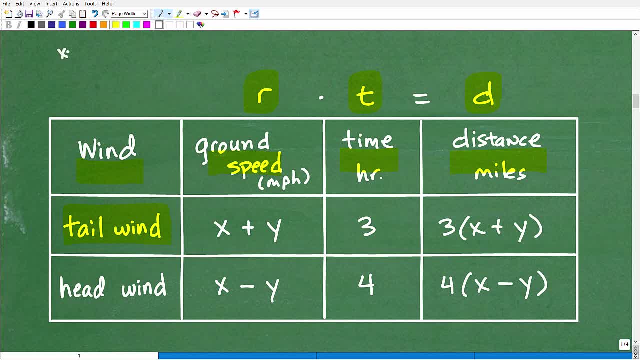 right. so let's take a look at this one situation. we have a tailwind, so the tail- right. so let's take a look at this one situation. we have a tailwind, so the tail wind. remember X, X is the speed of the situation. we have a tailwind, so the tail wind, remember X, X is the speed of the airplane. okay, remember, I just established. 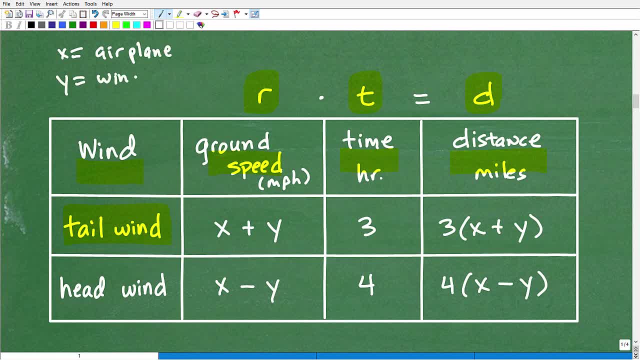 airplane. okay, remember, I just established airplane. okay, remember, I just established those variables, and Y is the wind speed. those variables, and Y is the wind speed. those variables, and Y is the wind speed. okay, all right. so the ground speed is okay, all right, so the ground speed is. 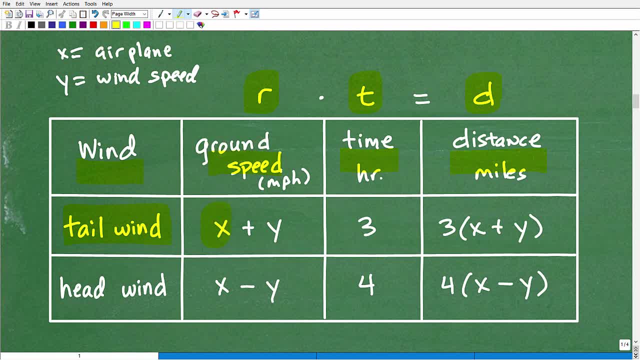 okay, all right. so the ground speed is kind of like the actual speed of the kind of like the actual speed of the kind of like the actual speed of the aircraft. so here, if my airplane is going aircraft, so here, if my airplane is going aircraft, so here, if my airplane is going X and I have a tailwind, I'm gonna have. 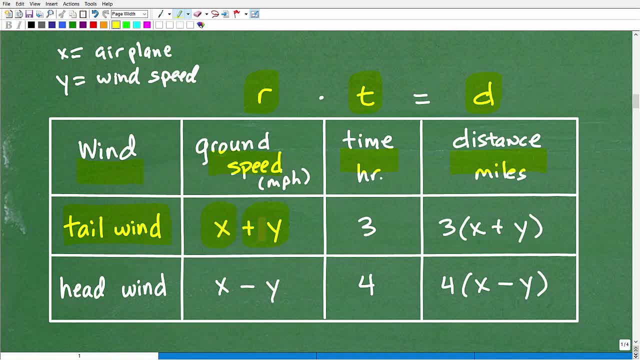 X and I have a tailwind. I'm gonna have X and I have a tailwind. I'm gonna have an additional like speed added to my you, an additional like speed added to my you, an additional like speed added to my, you know, actual ground speed, so it's gonna. 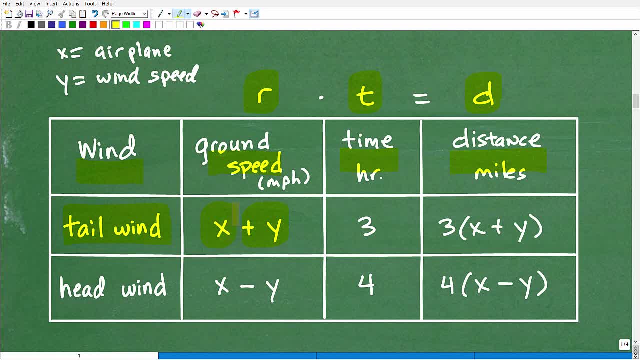 know actual ground speed, so it's gonna know actual ground speed. so it's gonna be X plus Y, so I'm actually going faster. be X plus Y, so I'm actually going faster. be X plus Y, so I'm actually going faster. okay, so the rate all right. when I have a 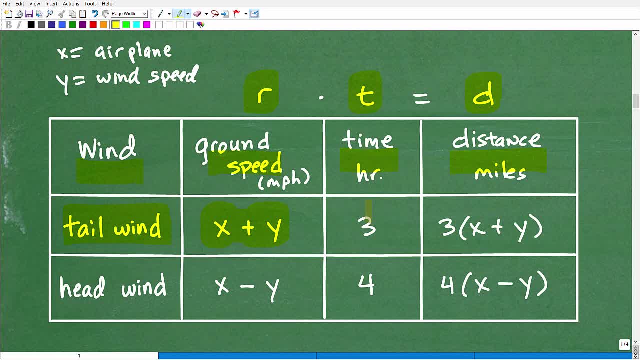 okay, so the rate all right when I have a. okay, so the rate all right when I have a tailwind is gonna be X plus Y. the time tailwind is gonna be X plus Y. the time tailwind is gonna be X plus Y. the time okay when I have the tailwind. remember. 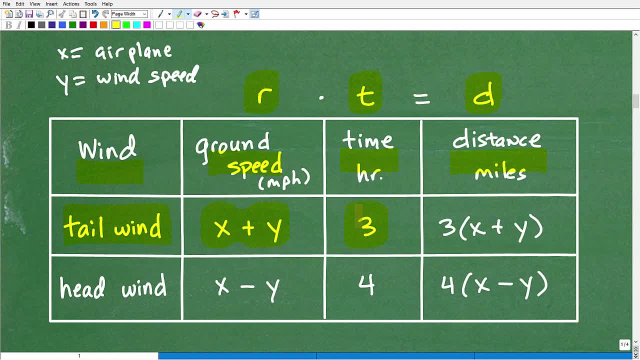 okay when I have the tailwind. remember, okay, when I have the tailwind. remember from the problem was three hours. okay, I from the problem was three hours. okay, I from the problem was three hours. okay, I was able to travel three hours. now the was able to travel three hours. now the. 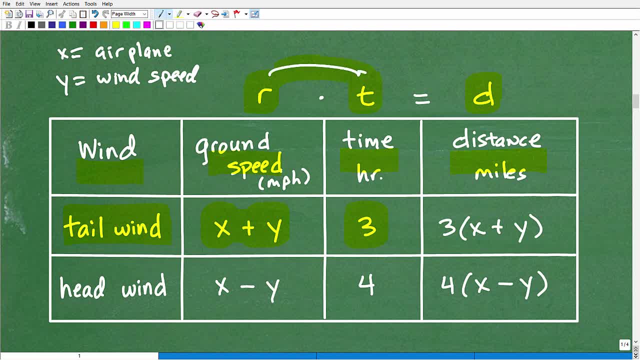 was able to travel three hours. now the rate times the time: all right rate rate times the time- all right rate rate times the time- all right rate times. time is equal to distance, so here my times time is equal to distance. so here my times time is equal to distance. so here my rate again is X plus Y, and I want to 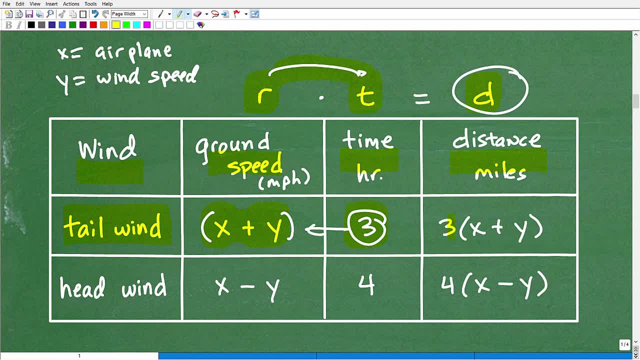 rate again is X plus Y and I want to rate again is X plus Y and I want to multiply it by three. okay, that is my multiply it by three. okay, that is my multiply it by three. okay, that is my distance. so it's gonna be three times X. 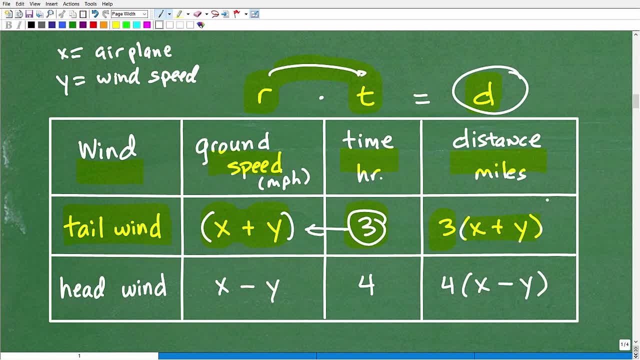 distance. so it's gonna be three times X distance. so it's gonna be three times X plus Y. now some of you might have been plus Y. now some of you might have been plus Y. now some of you might have been like, oh, isn't that 960? yeah, we don't. 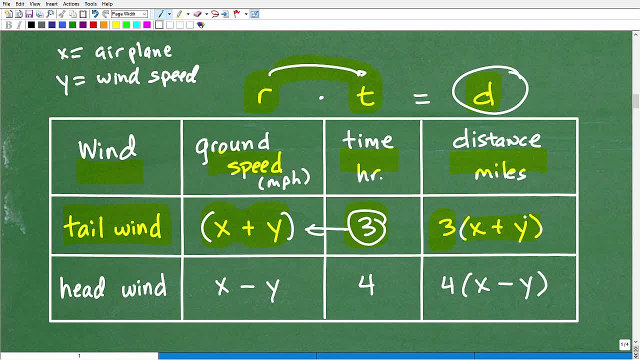 like: oh, isn't that 960? yeah, we don't like: oh, isn't that 960? yeah, we don't want to put that into our table right. want to put that into our table right, want to put that into our table right here. we want to use our variables first. 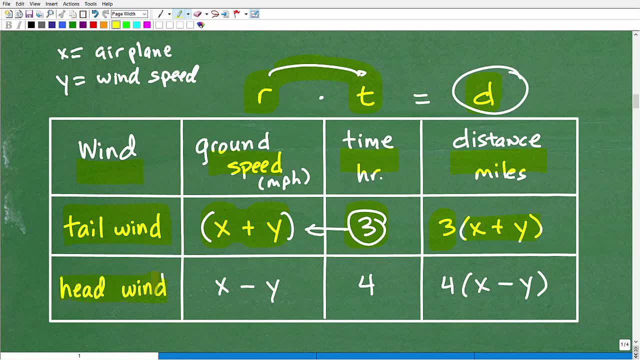 here we want to use our variables first. here we want to use our variables first. okay, now it's going to talk about a. okay, now it's going to talk about a. okay, now it's going to talk about a headwind. now, headwind, we go, our actual. 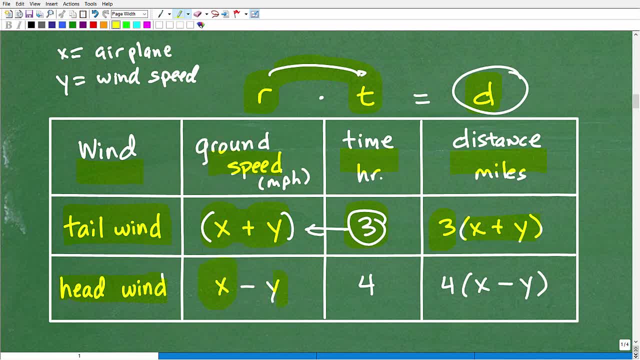 headwind, now headwind we go. our actual headwind, now headwind we go. our actual ground speeds gonna be slower. so it's ground speeds gonna be slower. so it's ground speeds gonna be slower. so it's the speed of the aircraft minus the wind, the speed of the aircraft minus the wind. 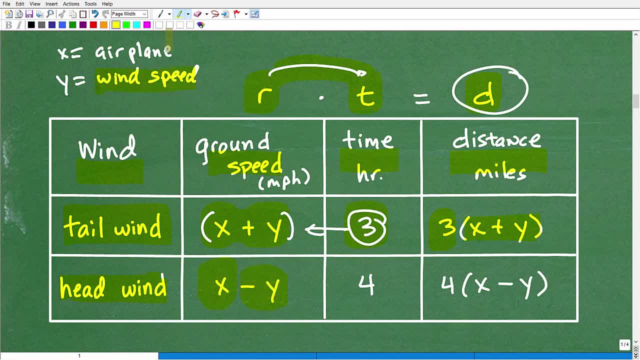 the speed of the aircraft minus the wind. now the wind is going into us, so we're now the wind is going into us, so we're now the wind is going into us, so we're gonna be going slower. so the time it gonna be going slower, so the time it. 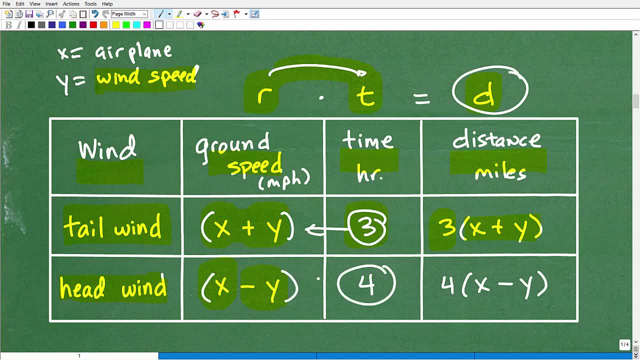 gonna be going slower. so the time it took for us to travel was four hours. took for us to travel was four hours. took for us to travel was four hours. okay, but the distance is still rate. okay, but the distance is still rate. okay, but the distance is still rate times time, so it's gonna be four times. 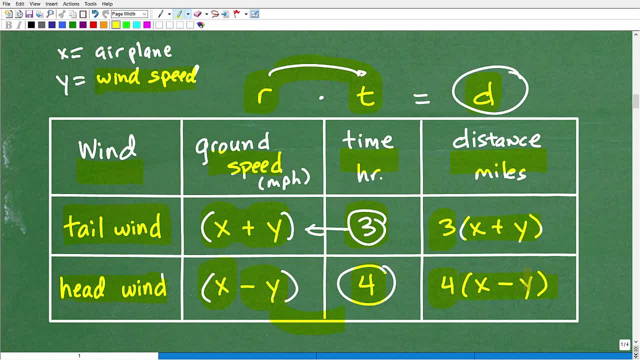 times time, so it's gonna be four times times time, so it's gonna be four times. it's X minus Y, so that's gonna be four. it's X minus Y, so that's gonna be four. it's X minus Y, so that's gonna be four times X minus Y. okay, now I'm hopefully. 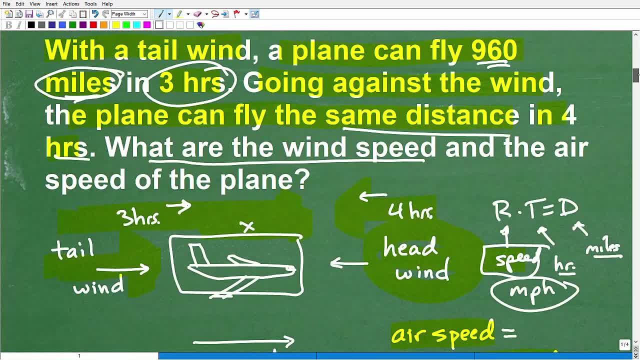 times X minus Y. okay, now I'm hopefully times X minus Y. okay, now I'm, hopefully. let's go back to the prom here. we know let's go back to the prom here. we know, let's go back to the prom here. we know that the distance travel was 960 miles. 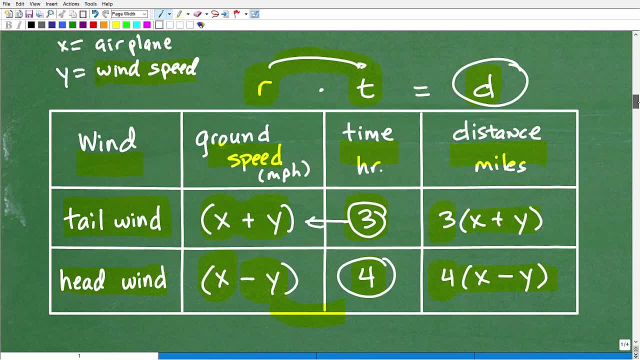 that the distance travel was 960 miles, that the distance travel was 960 miles. okay, so this distance right here. this okay, so this distance right here, this okay. so this distance right here, this distance with the tailwind and this distance with the tailwind, and this. 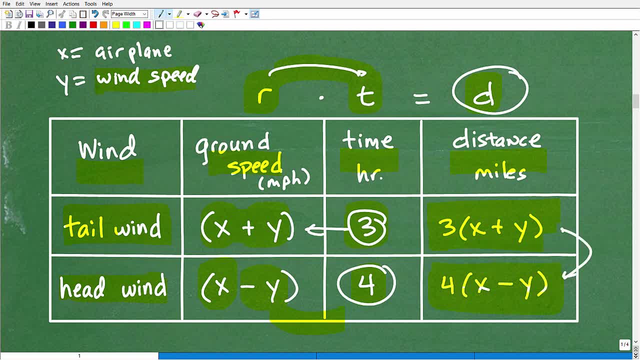 distance with the tailwind and this distance, they're the same. okay, both of distance they're the same. okay, both of distance they're the same. okay. both of these right here are 960 miles, so we can. these right here are 960 miles, so we can. 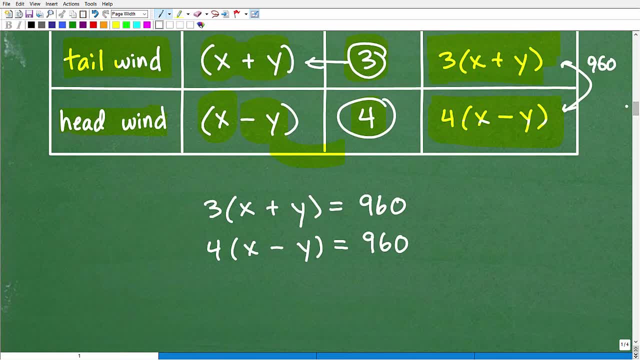 these right here are 960 miles, so we can use this table here to construct, use this table here to construct, use this table here to construct formulas, all right, so here we have 3 formulas. all right, so here we have 3 formulas. all right, so here we have 3 times X plus Y that distance. that's what. 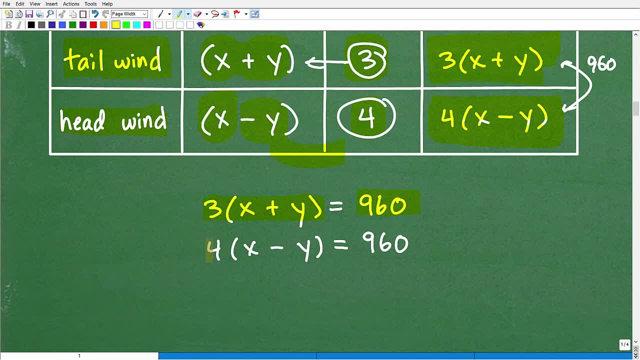 times X plus Y that distance, that's what. times X plus Y that distance, that's what. that's equal to 960 miles, and 4 times X that's equal to 960 miles. and 4 times X that's equal to 960 miles. and 4 times X minus Y, that's the distance with the 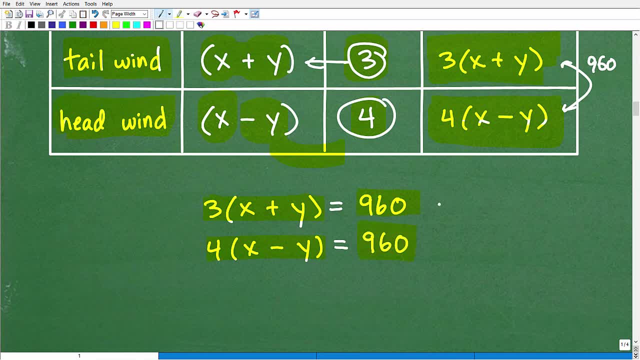 minus Y. that's the distance with the minus Y. that's the distance with the headwind. that's also equal to 960 miles. headwind- that's also equal to 960 miles headwind- that's also equal to 960 miles. so now, what do I have here? all right, 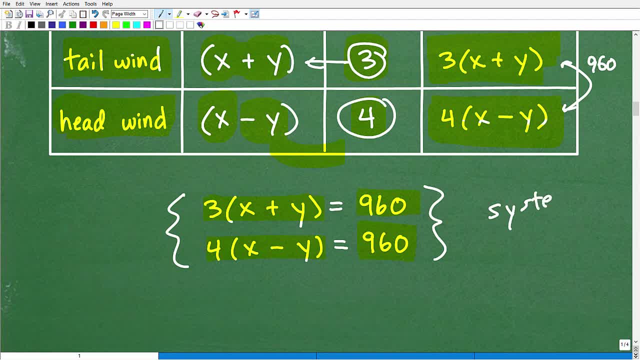 so now, what do I have here? all right. so now, what do I have here? all right, well, I have a basic system, okay, system. well, I have a basic system, okay system. well, I have a basic system, okay, system of equations, because I have both X and Y. 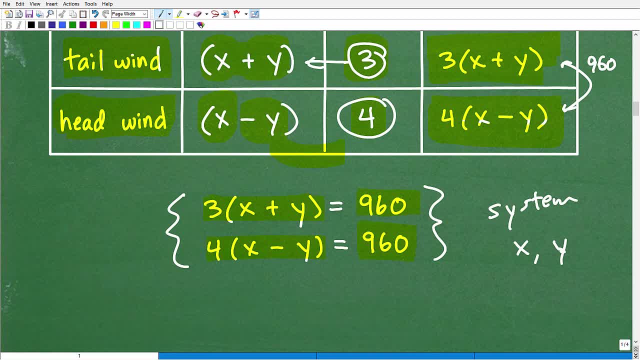 of equations because I have both X and Y of equations because I have both X and Y, are as variables I need to solve for now. are as variables I need to solve for now. are as variables I need to solve for now. another thing, another little tip here: 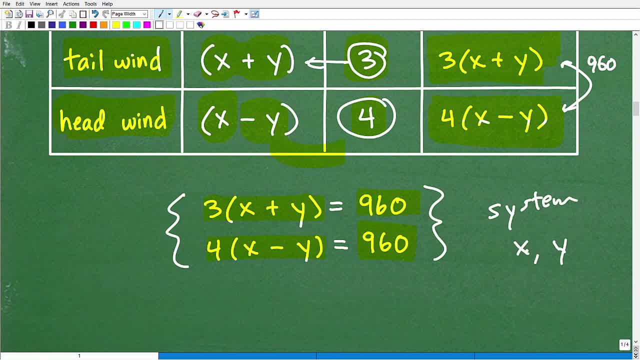 another thing, another little tip here. another thing, another little tip here is when you have more than one variable, the is when you have more than one variable. the is, when you have more than one variable, the amount of variables you have in your, amount of variables you have in your. 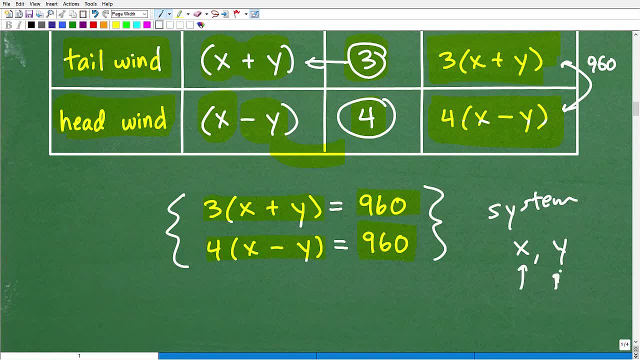 amount of variables you have in your problem. here I have two. I have an X and a problem. here I have two. I have an X and a problem. here I have two. I have an X and a Y. I'm gonna need at least two separate Y. I'm gonna need at least two separate. 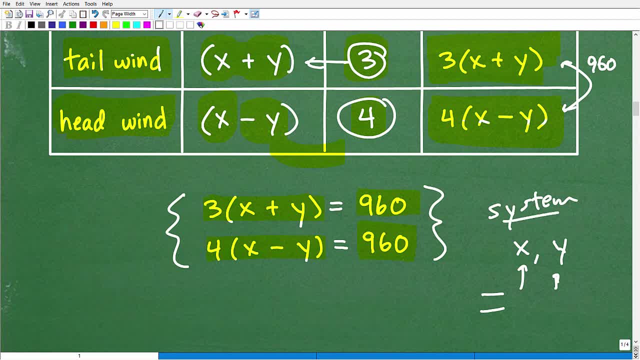 Y, I'm gonna need at least two separate equations. okay, that's kind of a general equations. okay, that's kind of a general equations. okay, that's kind of a general rule. so we're talking about a system I rule. so we're talking about a system I. 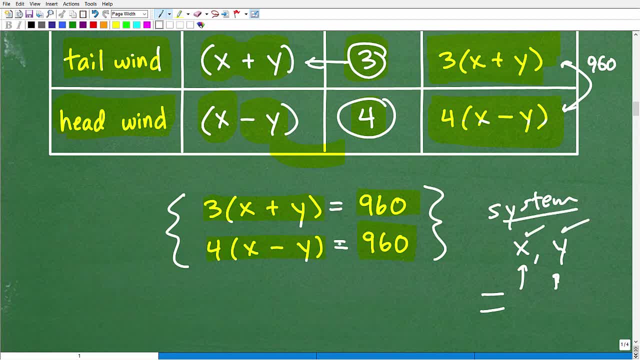 rule. so we're talking about a system. I have an X and a Y, so I need to have two. have an X and a Y, so I need to have two. have an X and a Y, so I need to have two, two equations to solve for both X and Y. 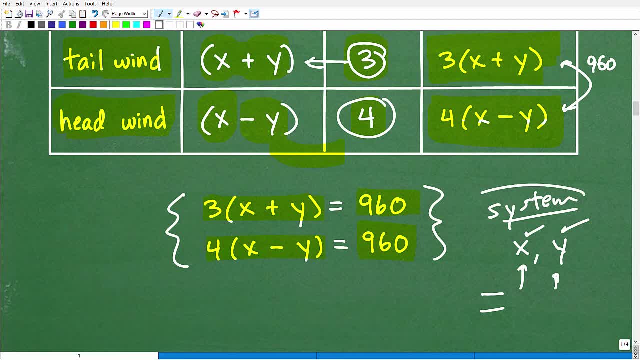 two equations to solve for both X and Y. two equations to solve for both X and Y. and this is it so now, if I can solve for, and this is it so now if I can solve for, and this is it so now, if I can solve for X and Y here, and that is going to be. 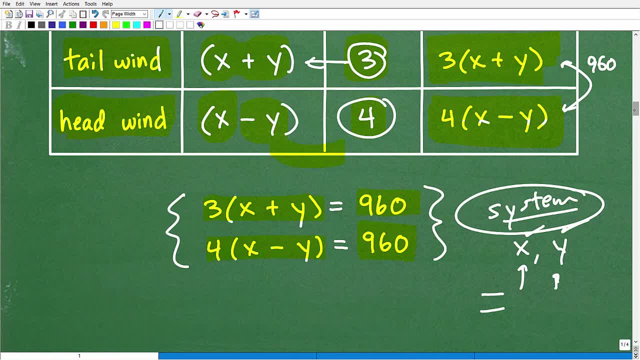 X and Y here, and that is going to be X and Y here, and that is going to be dependent upon my knowledge of systems, dependent upon my knowledge of systems, dependent upon my knowledge of systems. okay. so again, algebra, word problems you. okay. so again, algebra, word problems you. 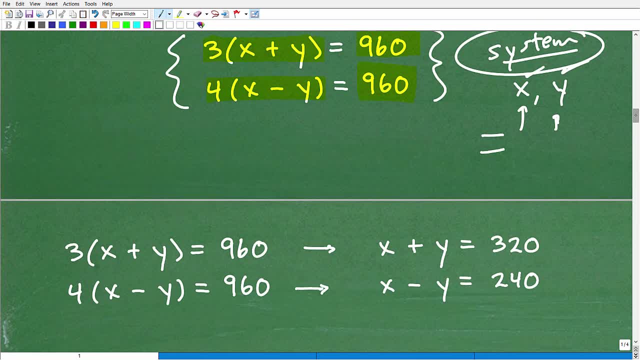 okay, so again, algebra word problems, you know, involve all the things that you know, involve all the things that you know, involve all the things that you should be learning- all the sub skills- but should be learning all the sub skills, but should be learning all the sub skills. but let's go ahead and now solve this. 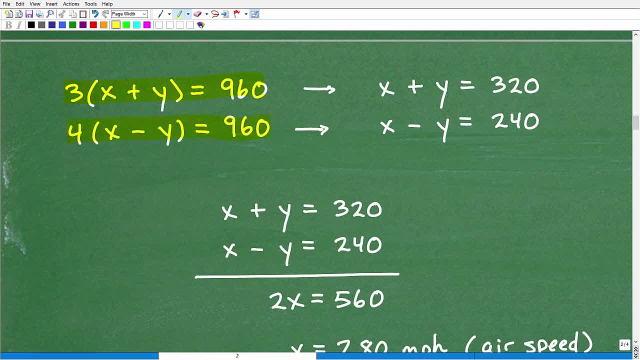 let's go ahead and now solve this. let's go ahead and now solve this system. all right, so we have. this was our system. all right, so we have. this was our system. all right, so we have. this was our original setup now here. notice: I have original setup now here. notice I have. 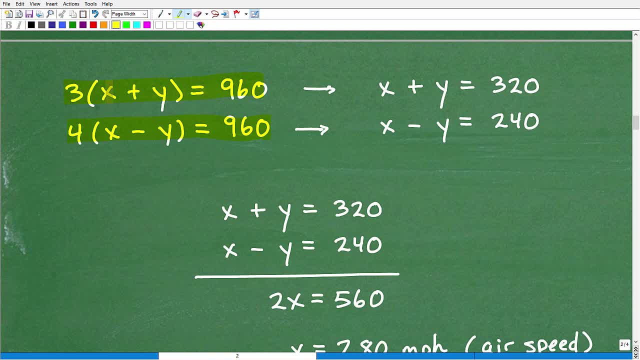 original setup. now here, notice, I have three times this thing right here, I three times this thing right here. I three times this thing right here. I could divide both sides of the equation, could divide both sides of the equation, could divide both sides of the equation by three and simplify the system. so 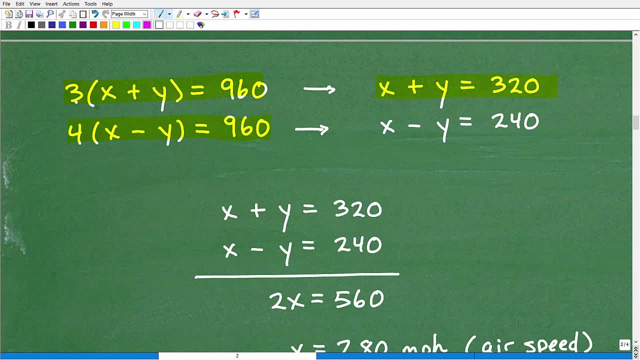 by three and simplify the system. so by three and simplify the system. so that's going to be: X plus Y is equal to. that's going to be. X plus Y is equal to. that's going to be: X plus Y is equal to 320. okay, so in other words, I have this: 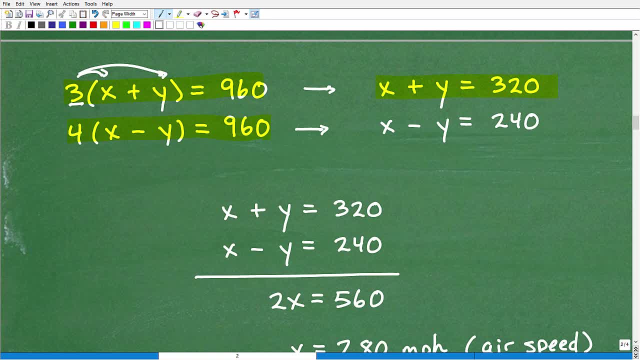 320. okay. so in other words, I have this 320. okay. so in other words, I have this three. I don't have to multiply like that three. I don't have to multiply like that three. I don't have to multiply like that. I could just be like: okay, divide both. 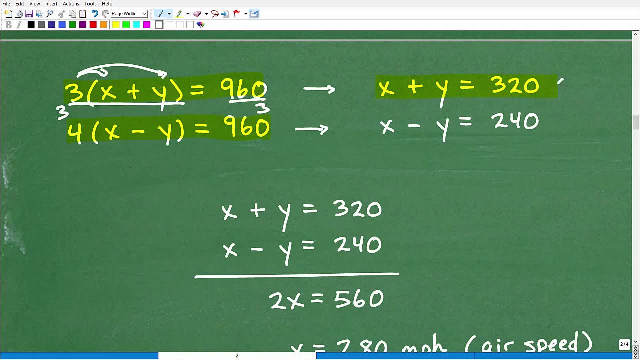 I could just be like: okay, divide both. I could just be like: okay, divide both sides of the equation by three, and let's sides of the equation by three, and let's sides of the equation by three, and let's just work with this simpler equation. just work with this simpler equation. 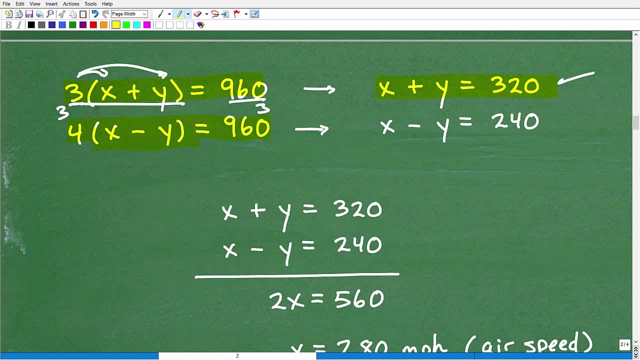 just work with this simpler equation there and then I'll divide both sides there, and then I'll divide both sides there, and then I'll divide both sides of the equation by four, and I got this of the equation by four, and I got this of the equation by four and I got this simpler version right there. so now this: 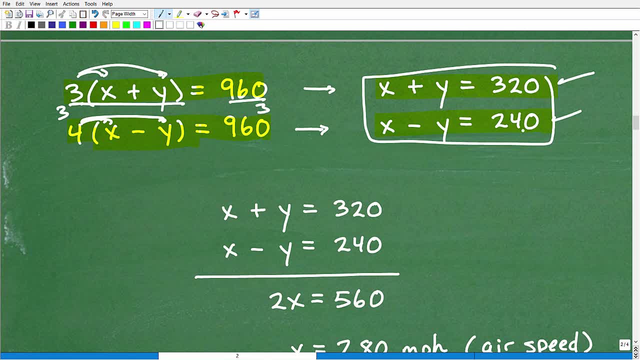 simpler version right there. so now this simpler version right there. so now this X plus Y is equal to 320 and X minus Y is. X plus Y is equal to 320 and X minus Y is X plus Y is equal to 320 and X minus Y is equal to 240. let's go ahead and solve. 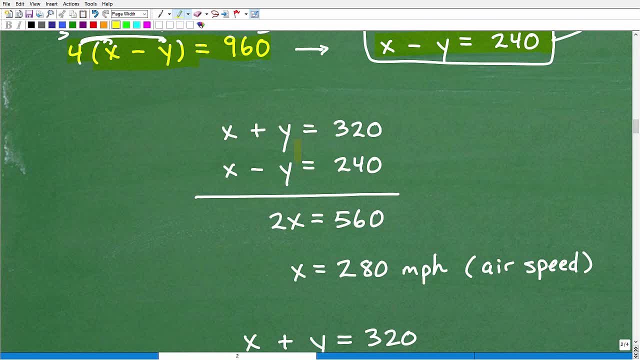 equal to 240, let's go ahead and solve equal to 240. let's go ahead and solve for X and Y and hopefully, if you're for X and Y, and hopefully if you're for X and Y and hopefully if you're really up to speed on solving systems. 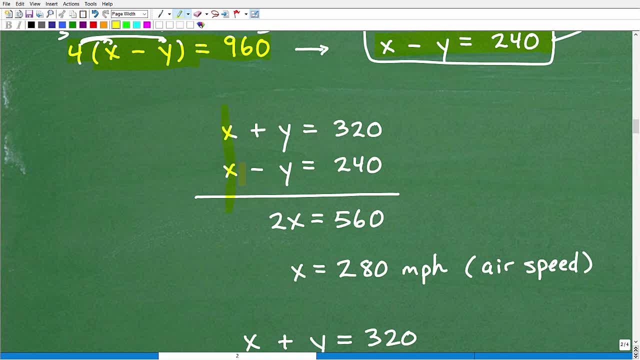 really up to speed on solving systems, really up to speed on solving systems, and you need to be to handle this and you need to be to handle this and you need to be to handle this particular problem. you can see I could. particular problem. you can see I could. 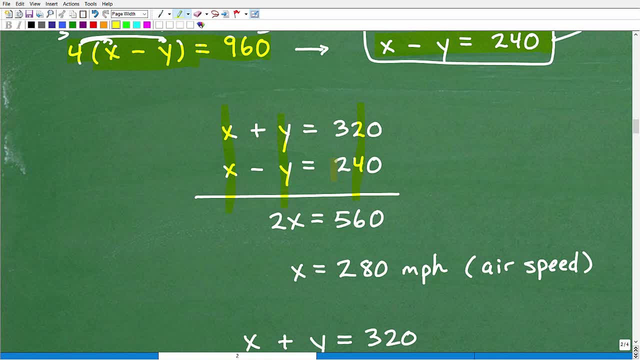 particular problem. you can see, I could just do the elimination method. I could just do the elimination method. I could just do the elimination method. I could just add these two down, or add these two. just add these two down, or add these two. just add these two down or add these two equations together. by the way, if you're 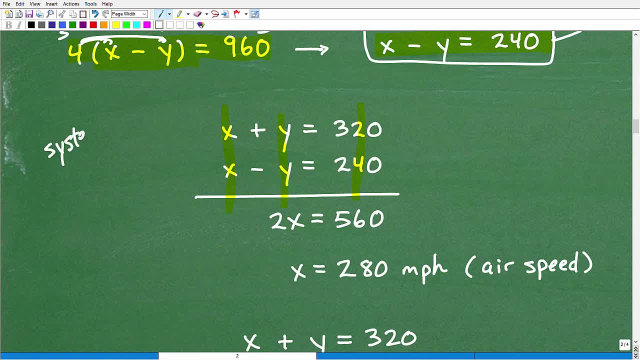 equations together. by the way, if you're equations together, by the way, if you're not quite sure what's going on here, you not quite sure what's going on here, you not quite sure what's going on here, you need to look at my additional videos on. 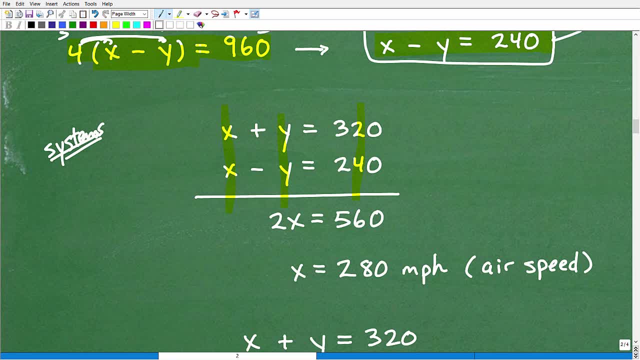 need to look at my additional videos on. need to look at my additional videos on systems. or, better yet, just go into my systems. or, better yet, just go into my systems. or, better yet, just go into my Algebra 1 course in my math help program. Algebra 1 course in my math help program. 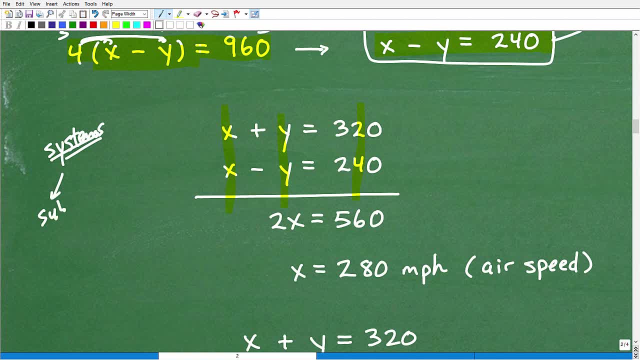 Algebra 1 course in my math help program. but you can use a substitution method. but you can use a substitution method. but you can use a substitution method here, or the elimination or linear here, or the elimination or linear here, or the elimination or linear combination method. I have tons of videos. 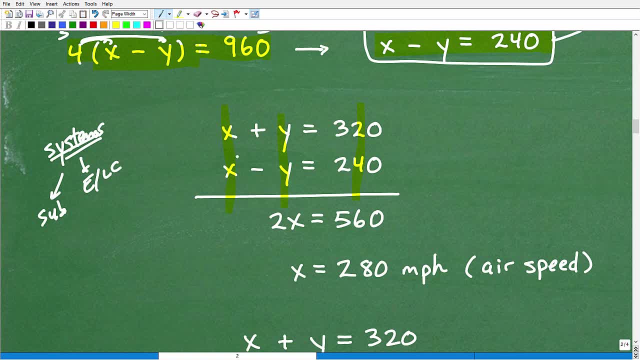 combination method. I have tons of videos, combination method. I have tons of videos on that in my youtube channel, in my on that in my youtube channel, in my on that in my youtube channel, in my algebra playlist. so if you're having algebra playlist, so if you're having 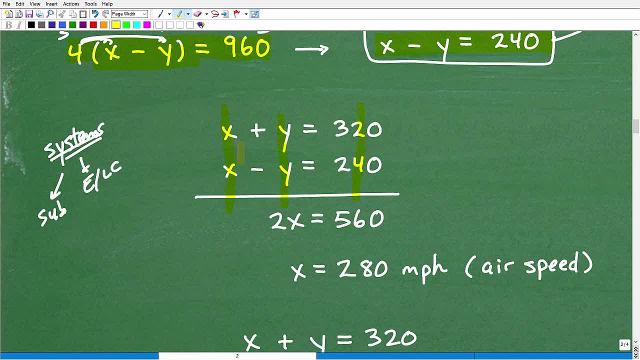 algebra playlist. so if you're having trouble with this algebra, check that. trouble with this algebra, check that. trouble with this algebra, check that stuff out. alright. so here I have X plus stuff out. alright. so here I have X plus stuff out. alright. so here I have X plus X. that's 2x. the Y's are eliminated plus. 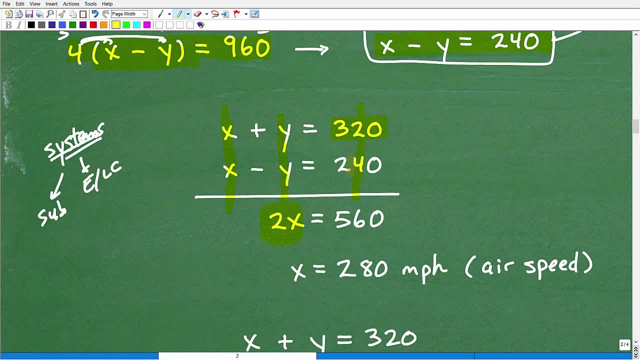 X, that's 2x, the Y's are eliminated. plus X, that's 2x, the Y's are eliminated. plus Y and negative Y, that's 0 Y, those go Y. and negative Y, that's 0 Y, those go Y. and negative Y, that's 0 Y, those go away. and the 320 and 320 and 240 is 560. away and the 320 and 320 and 240 is 560 away and the 320 and 320 and 240 is 560. so I have: 2x is equal to 560, I can. so I have: 2x is equal to 560, I can. 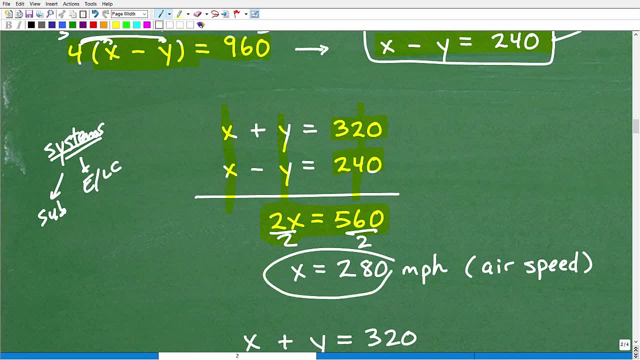 so I have: 2x is equal to 560. I can divide both sides of the equation by 2. divide both sides of the equation by 2. divide both sides of the equation by 2, so that gives me X is equal to 280. now. 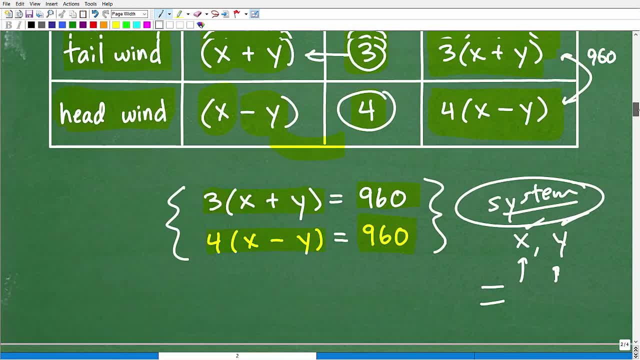 so that gives me X is equal to 280 now. so that gives me X is equal to 280 now. what was X? okay, let's go back up here. what was X? okay, let's go back up here. what was X? okay, let's go back up here and remember: X was the speed of the. 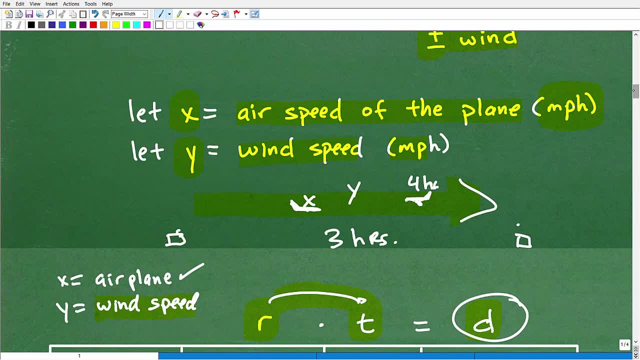 and remember X was the speed of the and remember X was the speed of the airplane in miles per hour, right way. airplane in miles per hour, right way. airplane in miles per hour, right way back here. remember we let X equal the back here. remember we let X equal the. 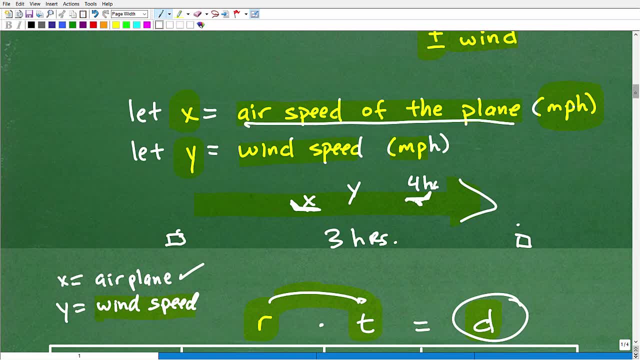 back here. remember we let X equal the. that's the air speed of the plane in. that's the air speed of the plane in. that's the air speed of the plane in miles per hour. okay, so we got that now. miles per hour: okay, so we got that now. 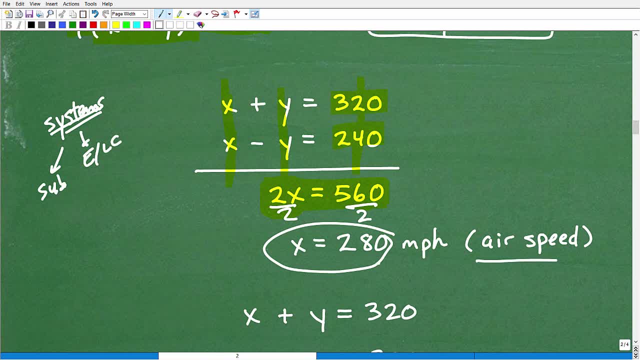 miles per hour. okay, so we got that now. okay, so the airplane its airspeed is okay. so the airplane its airspeed is okay. so the airplane its airspeed is 280 miles per hour. now I need to solve. 280 miles per hour, now I need to solve. 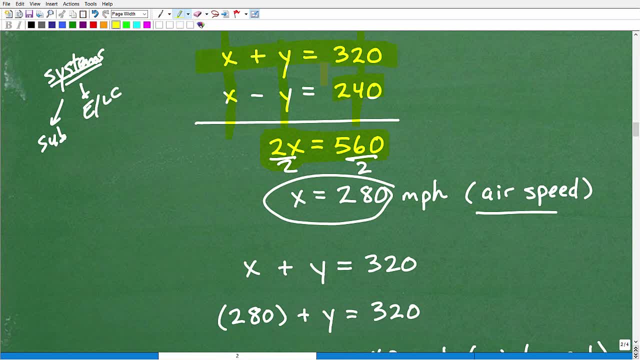 280 miles per hour. now I need to solve for Y. so when I'm solving for Y, I can for Y. so when I'm solving for Y, I can for Y. so when I'm solving for Y, I can use any one of these equations right. use any one of these equations right. 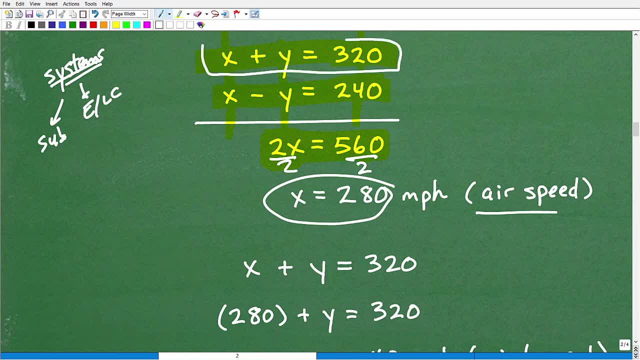 use any one of these equations right here. so let's say, I'll use this equation here. so let's say I'll use this equation here. so let's say, I'll use this equation: X plus Y is equal to 320. okay, X plus Y. X plus Y is equal to 320. okay, X plus Y. 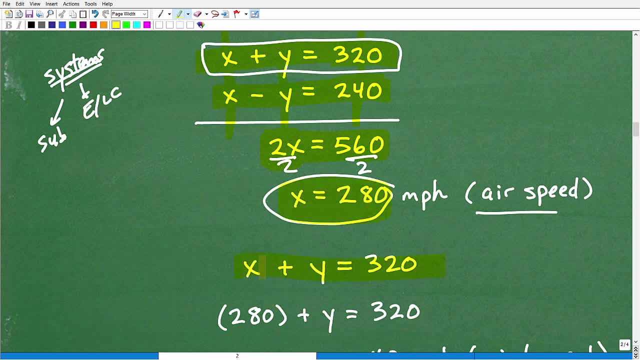 X plus Y is equal to 320. okay, X plus Y is equal to 320. so now that I know that is equal to 320, so now that I know that is equal to 320, so now that I know that X is equal to 280, I can just replace. 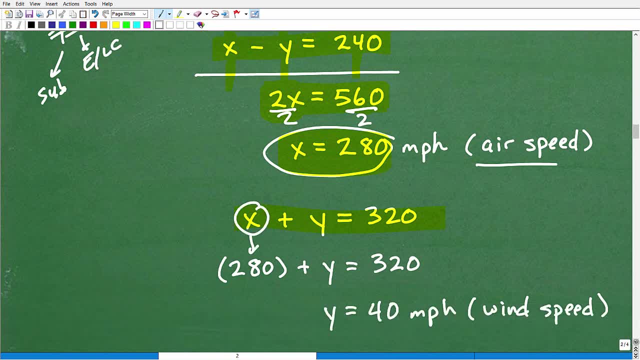 X is equal to 280. I can just replace: X is equal to 280. I can just replace this X with 280 and solve for Y- okay. so this X with 280 and solve for Y- okay. so this X with 280 and solve for Y- okay, so let's go ahead and do that now. so 280. 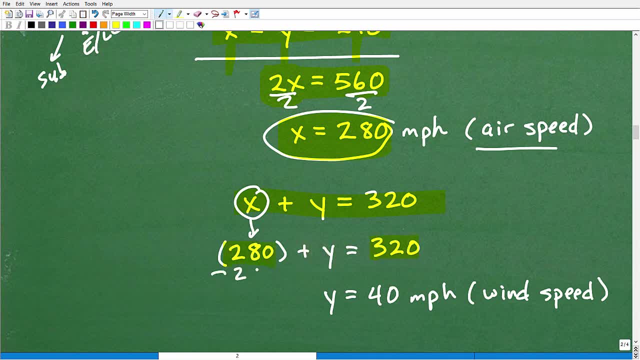 let's go ahead and do that now. so 280. let's go ahead and do that now. so 280 plus Y is equal to 320. I'm gonna go plus Y is equal to 320. I'm gonna go plus Y is equal to 320. I'm gonna go ahead and subtract 280 from both sides of. 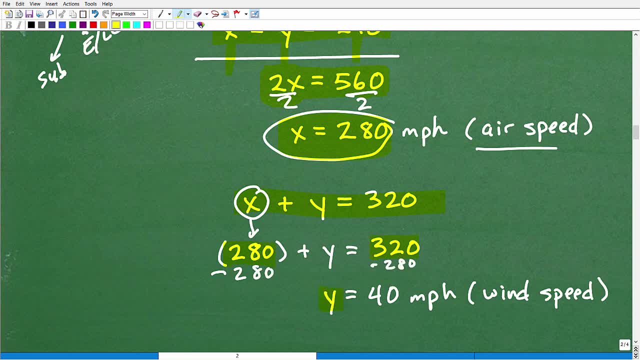 ahead and subtract 280 from both sides of ahead and subtract 280 from both sides of the equation, and that gives me Y is the equation, and that gives me Y is the equation, and that gives me Y is equal to 40, okay, or 40 miles per hour. 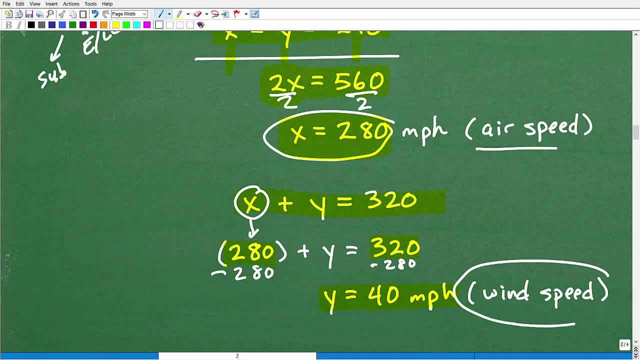 equal to 40- okay, or 40 miles per hour. equal to 40- okay, or 40 miles per hour. and if you recall that was the wind and if you recall that was the wind and if you recall that was the wind speed. so the airplane is going 280. 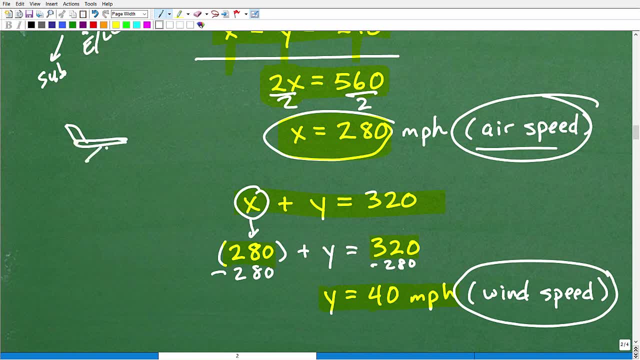 speed. so the airplane is going 280 speed. so the airplane is going 280 miles per hour. so here's our little plane, miles per hour. so here's our little plane, miles per hour. so here's our little plane right here: it's going 280 miles per. 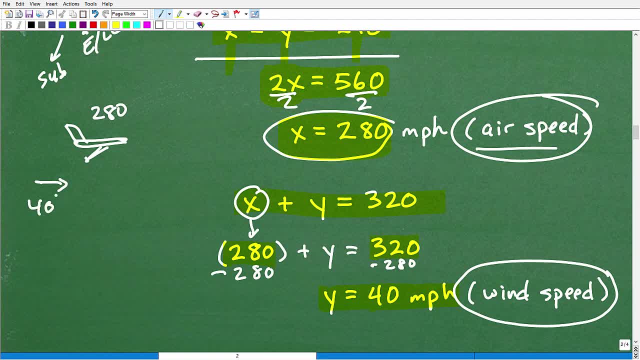 right here it's going 280 miles per right. here it's going 280 miles per hour and the wind is going 40- okay hour and the wind is going 40- okay hour and the wind is going 40- okay, sometimes it's going 40 as a tailwind or. 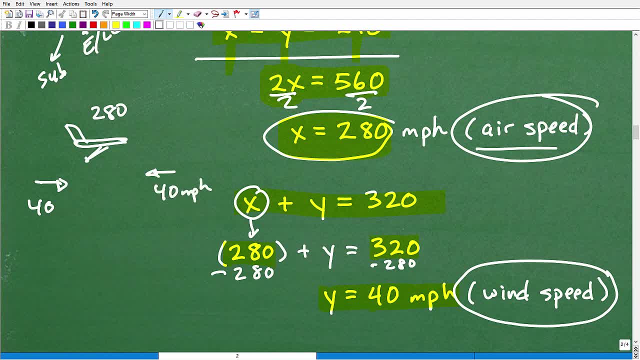 sometimes it's going 40 as a tailwind, or sometimes it's going 40 as a tailwind, or it's going 40 miles per hour as a. it's going 40 miles per hour as a. it's going 40 miles per hour as a headwind- okay, but the airplane is at 280. 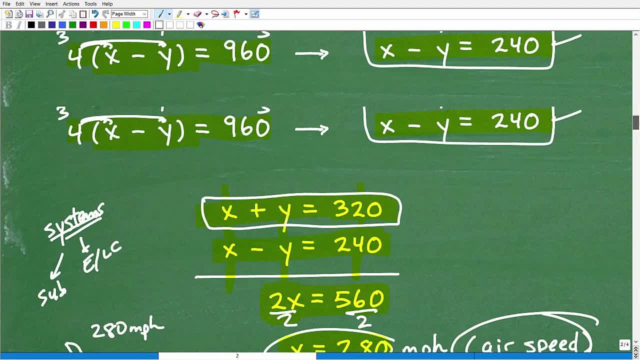 headwind okay, but the airplane is at 280. headwind okay, but the airplane is at 280 miles per hour and that is it okay. so miles per hour and that is it okay. so miles per hour and that is it okay. so this particular problem, this is a little. 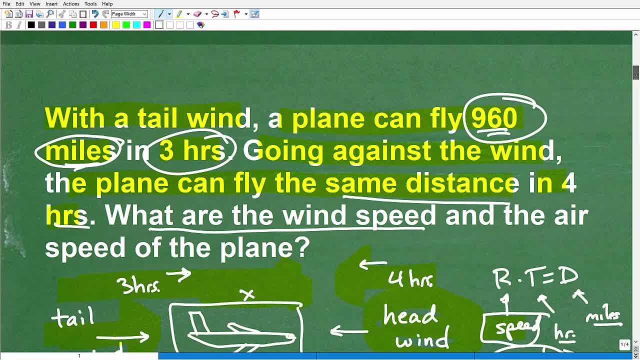 this particular problem. this is a little this particular problem. this is a little bit more involved because it didn't bit more involved, because it didn't bit more involved, because it didn't involve a system and there was two involve a system and there was two involve a system and there was two variables. and you know, this might be a 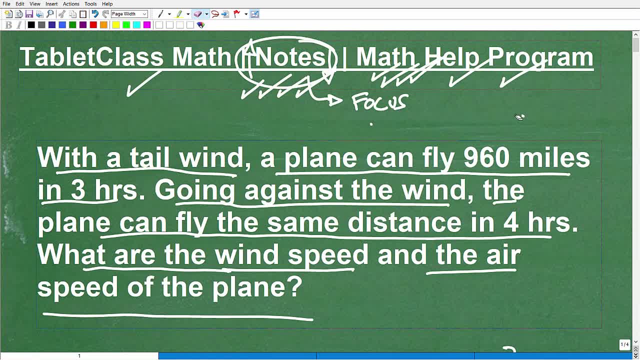 variables and you know this might be a variables and you know this might be a little bit, maybe a little advanced for little bit. maybe a little advanced for little bit, maybe a little advanced for some of you out there now, if you're some of you out there now, if you're. 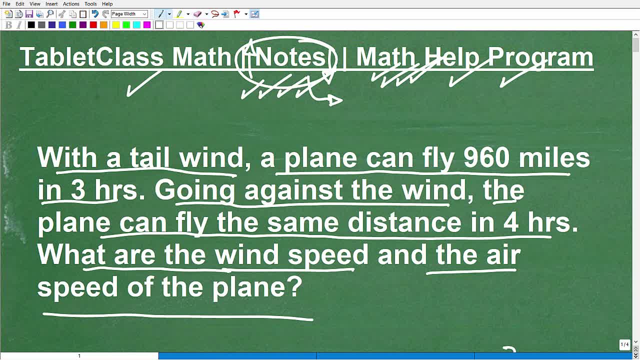 some of you out there now, if you're reviewing algebra and you're looking at reviewing algebra and you're looking at reviewing algebra and you're looking at word prompts, you might want to start word prompts. you might want to start word prompts. you might want to start with some simpler word prompts again. I 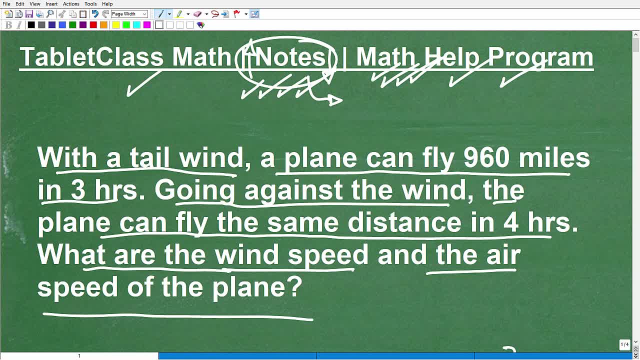 with some simpler word prompts again. I with some simpler word prompts again. I have multiple videos, different word. have multiple videos, different word. have multiple videos, different word. problems in my algebra playlist and problems in my algebra playlist and problems in my algebra playlist and pre-algebra playlist. so check those out. 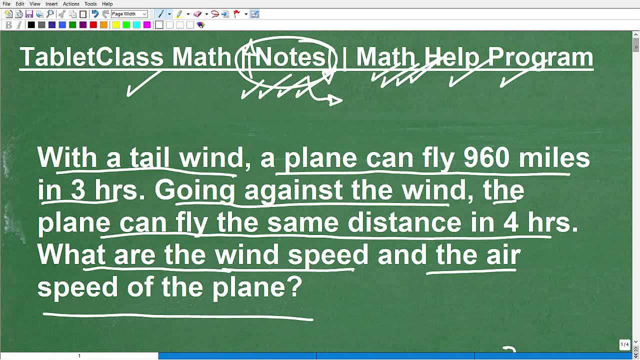 pre-algebra playlist, so check those out. pre-algebra playlist, so check those out as well. but the main idea again is as well. but the main idea again is as well, but the main idea again is always going to be this general, always going to be this general. 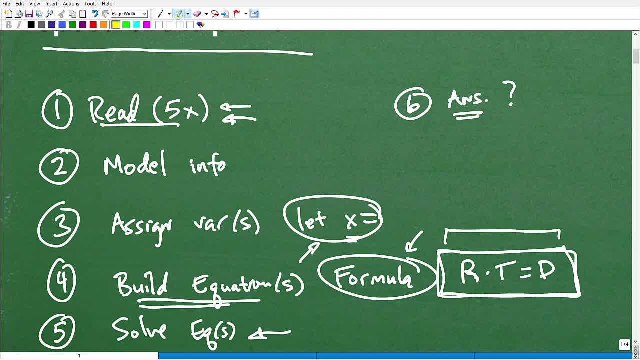 always going to be this general procedure: okay, read the prom, okay. model procedure. okay, read the prom, okay model procedure. okay, read the prom, okay. model the information. assign the variable or the information. assign the variable or the information. assign the variable or variables, build equations and, in order: 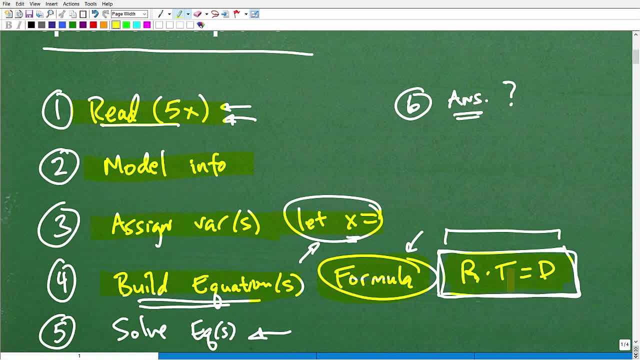 variables build equations. and, in order, variables build equations. and in order to build equations, you may need to know to build equations. you may need to know to build equations, you may need to know formulas like the ones we just talked, formulas like the ones we just talked, formulas like the ones we just talked about: rate times, times equal to distance. 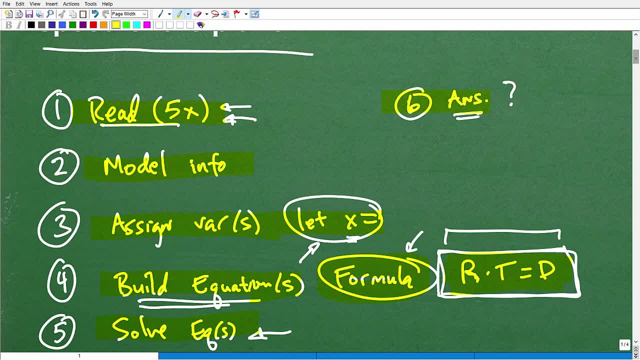 about rate times, times equal to distance, about rate times, times equal to distance. solve those equations and then make sure solve those equations and then make sure solve those equations and then make sure you answer the question appropriately. if you answer the question appropriately, if you answer the question appropriately, if you follow that those general guidelines, 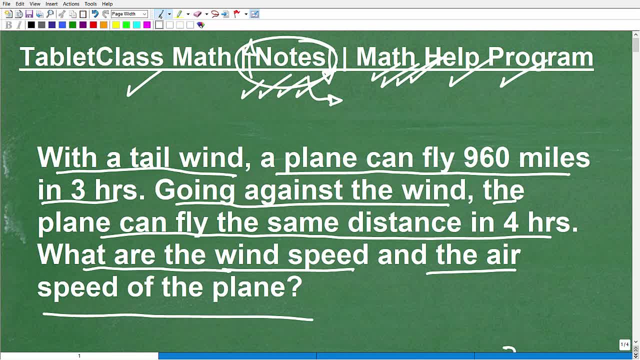 you follow that those general guidelines. you follow that those general guidelines. you're going to do very well with algebra. you're going to do very well with algebra. you're going to do very well with algebra. were problems okay, so hopefully this. were problems okay, so hopefully this. 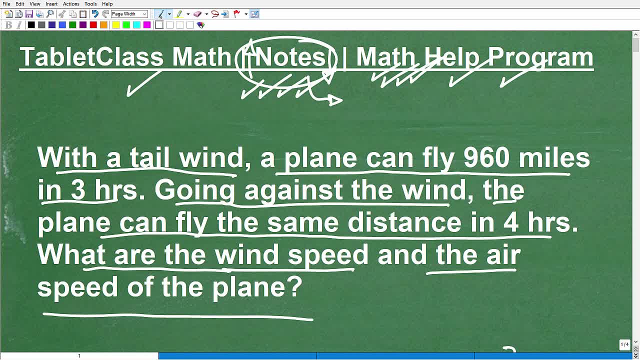 were problems, okay, so hopefully this problem was fun. okay, you're like, yeah, it problem was fun. okay, you're like, yeah, it problem was fun. okay, you're like, yeah, it was lots of fun. well, you know what I was fun. okay, you're like, yeah, it was lots of fun. well, you know what I. 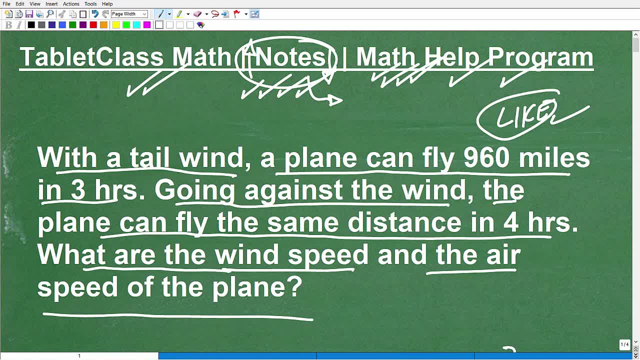 was fun. okay, you're like, yeah, it was lots of fun. well, you know what? I haven't been on YouTube for a. haven't been on YouTube for a. haven't been on YouTube for a long time. my goal is to teach math in a long time. my goal is to teach math in a. 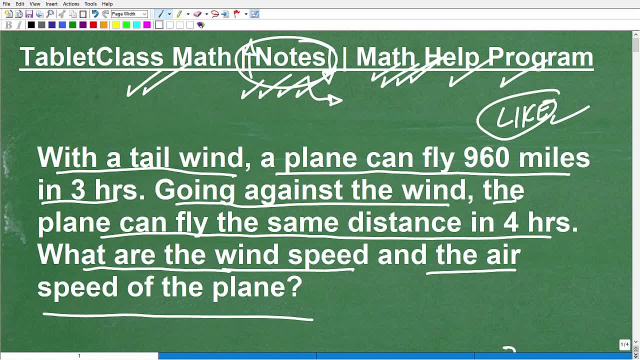 long time. my goal is to teach math in a clear and understandable way. okay, clear and understandable way. okay, clear and understandable way. okay, nobody should be failing math these days. nobody should be failing math these days. nobody should be failing math these days. if you're doing the right things, taking 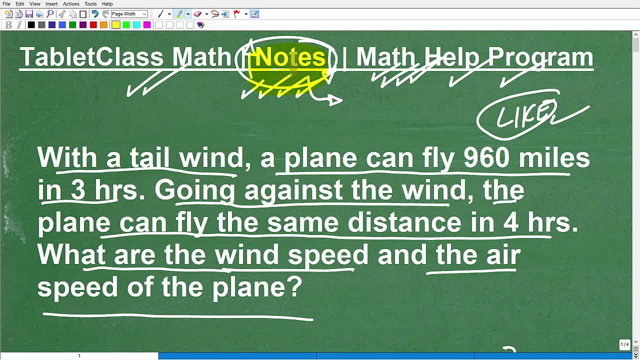 if you're doing the right things taking, if you're doing the right things taking notes. okay, there's a ton of free notes. okay, there's a ton of free notes. okay, there's a ton of free resources out there for you to go find, resources out there for you to go find. 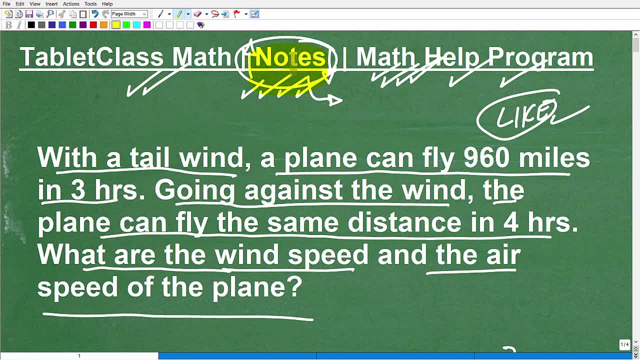 resources out there for you to go find the help that you need. okay, so there's a the help that you need. okay, so there's a the help that you need. okay, so, there's a ton of options if you like my teaching. ton of options if you like my teaching. 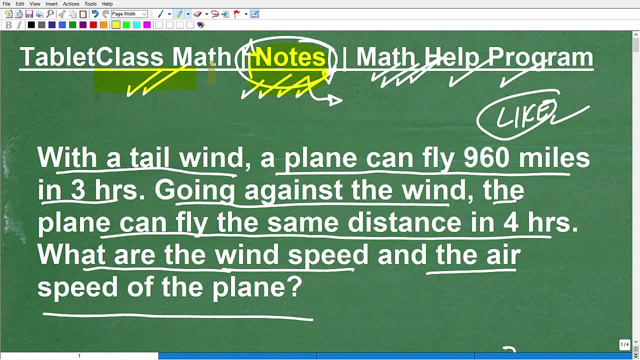 ton of options. if you like my teaching style, please take advantage of all the style. please take advantage of all the style. please take advantage of all the videos that I've made on my channel and videos that I've made on my channel and videos that I've made on my channel- and I'm making stuff all the time, so that's. 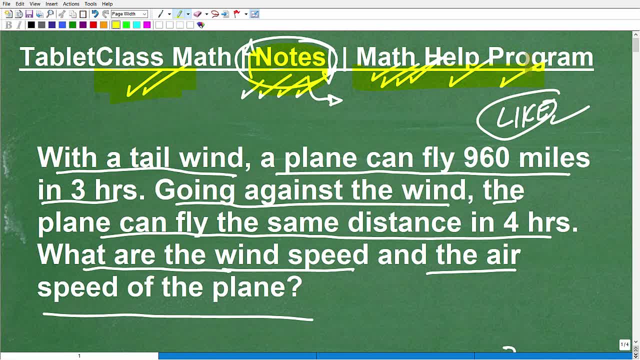 I'm making stuff all the time. so that's: I'm making stuff all the time. so that's why, hopefully you'll become a, why hopefully you'll become a, why hopefully you'll become a subscriber. but my best math help will subscriber, but my best math help will. 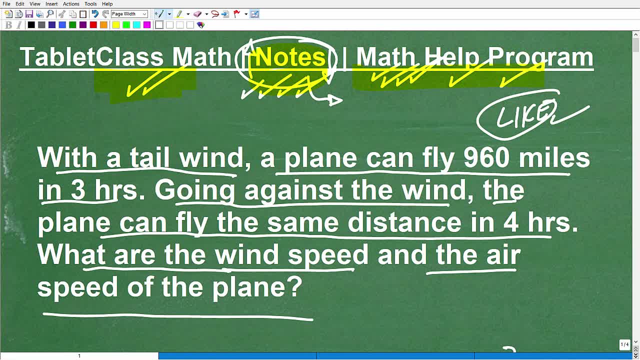 subscriber. but my best math help will always be within my math help program, always be within my math help program, always be within my math help program, okay? so, with that being said, I definitely okay. so, with that being said, I definitely okay. so, with that being said, I definitely wish you all the best in your 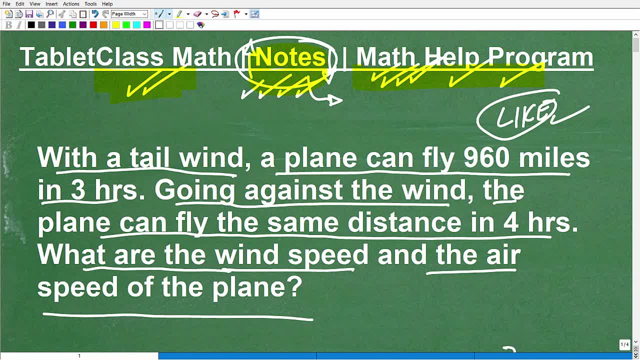 wish you all the best in your wish you all the best in your mathematics adventures. thank you for mathematics adventures. thank you for mathematics adventures. thank you for your time and have a great day.